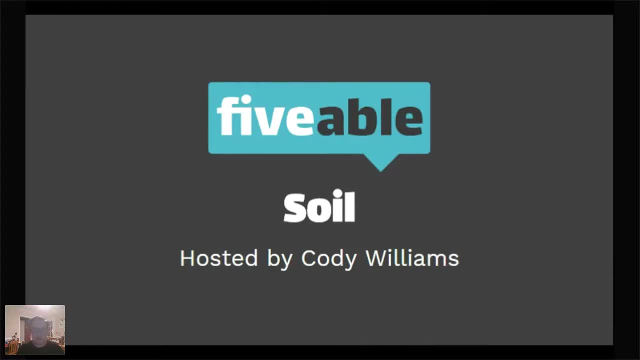 it's really a general topic. We're talking about formation of soil, the soil texture triangle, properties of soil, soil in different biomes, all those different kinds of things. So in the polls, tell me how you're doing, and also in the chat. 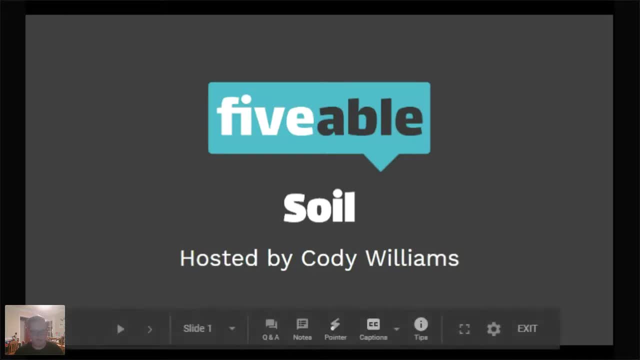 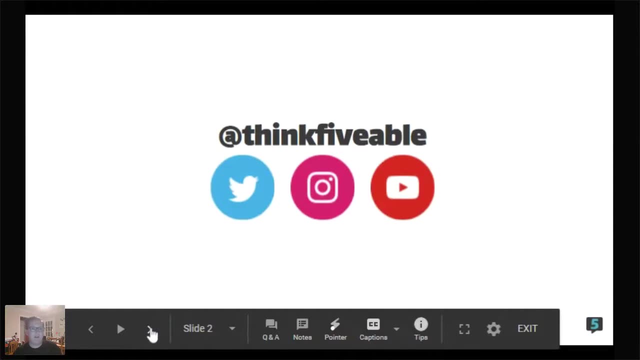 if there's anything particular that you might need help on, And feel free to ask questions Any time during the PowerPoint, All right, but more importantly, follow at ThinkFiveable on Instagram, Twitter and YouTube. Stay up to date on all the AP Environmental Science live streams so that you never miss out. 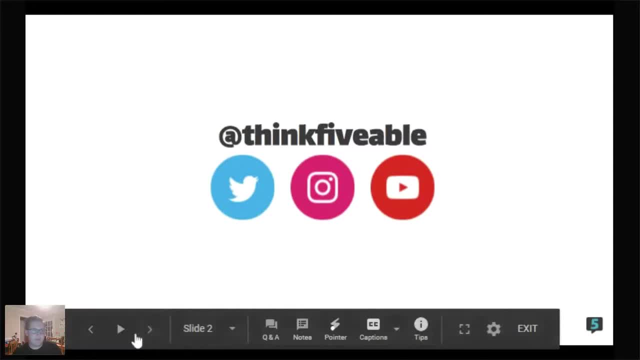 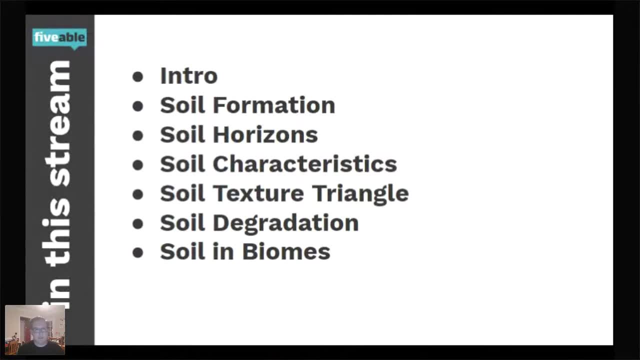 and you can review all the topics that you need to and know when live streams are happening. All right, so, as I mentioned before, in this live stream we're going to be talking about soil formation, soil horizons, soil characteristics. 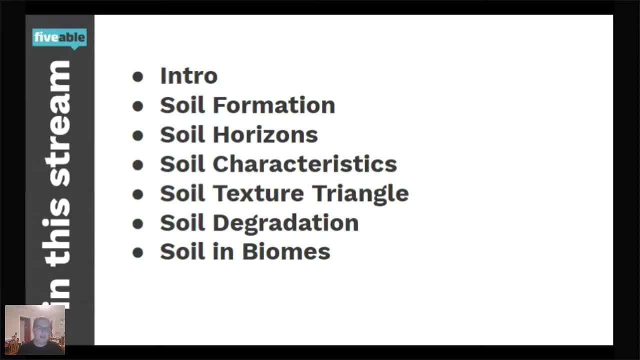 soil texture triangle, soil degradation and soil and biomes. So out of those there, which ones do you think you guys will need the most help with? Most difficult- It doesn't have to be like really difficult, but the most difficult items. 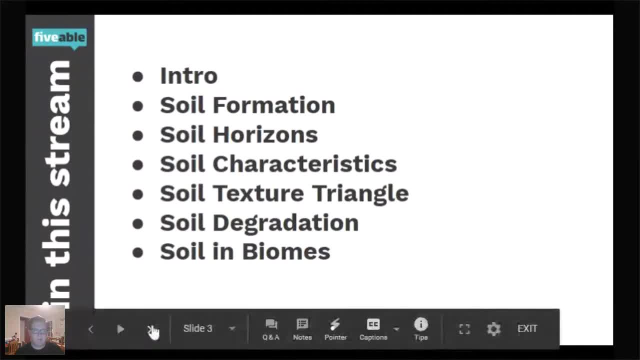 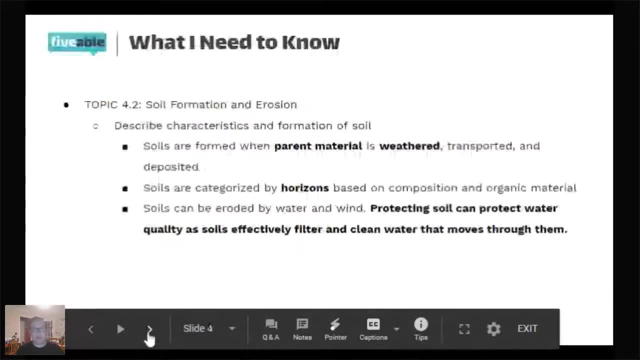 Send me on the chat. All right, On to our next slide. All right, so here is what I took from the CEF, CED: soil and biomes. All right, we'll cover that toward the end of the live stream, definitely. 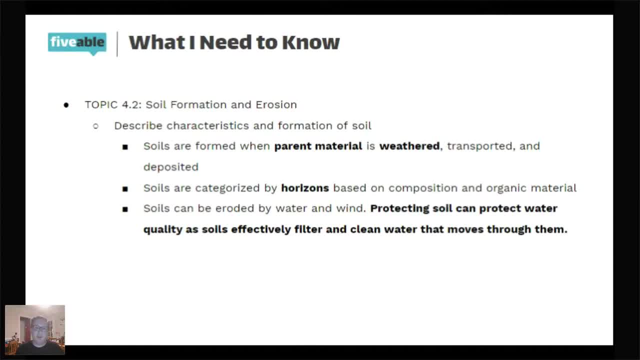 All right. so what is on here is basically what you need to know. This is from the AP Environmental Science course exam description, which is a great resource for studying for AP Environmental Science. It tells you everything you need to know and, particularly on this slide, what you need to. 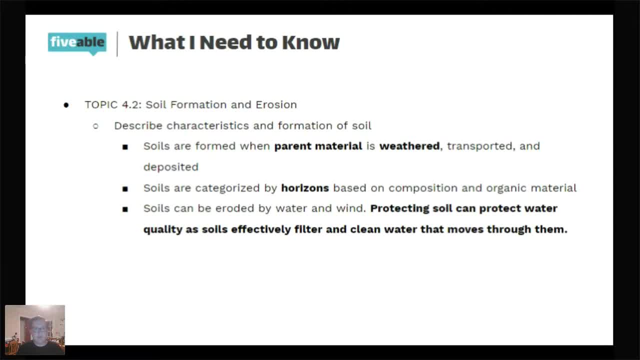 know about soil. Okay, so topic 4.2, if you want to check this, CED yourself: Soil formation and erosion. So, basically, what you need to understand is how to describe characteristics and formation of soil. It talks about parent material, like when it's weathered. 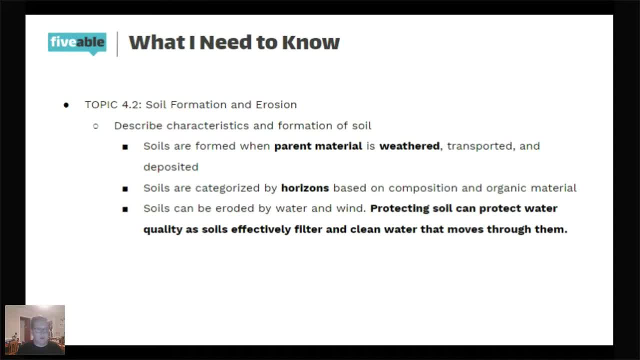 transported, deposited And then also looped into. this is soil horizons based on composition in terms of soil. So what you need to understand is how to describe characteristics and formation, And then also looped into this is soil horizons based on composition in terms of soil. So what you 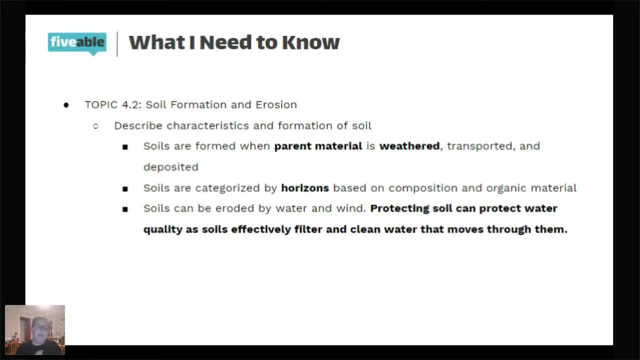 and organic matter, And then finally this one. I don't talk about a lot in this live stream, but protecting soil can protect water quality, as soils effectively filter and clean water that moves through them. I'll mention that a few times, but if you have any other, 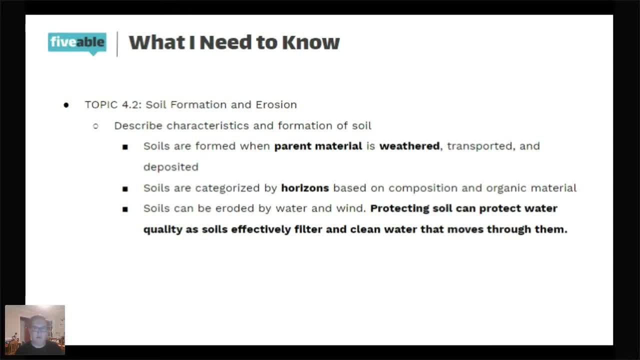 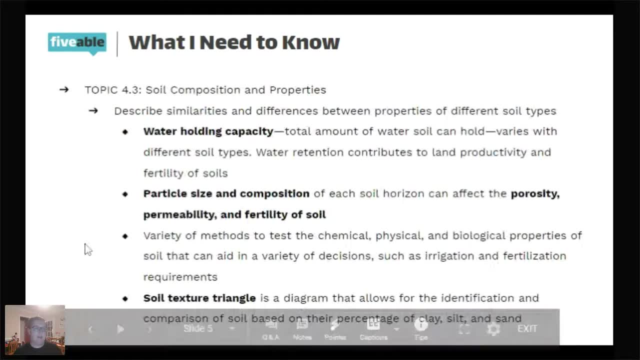 questions on that. just let me know after I'm finished or if you think of something during the live stream. And then also we have topic 4.3, soil composition and properties. water holding capacity, particle size and composition, porosity, permeability, fertility. 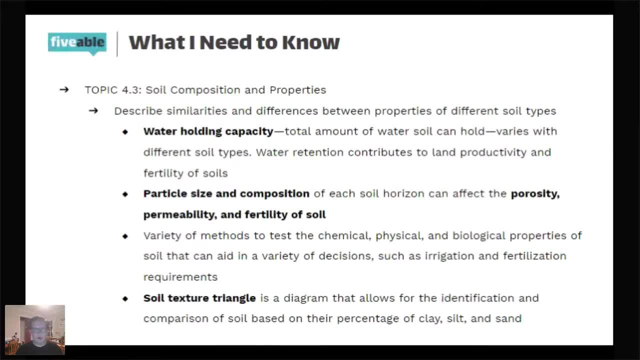 of soil, other chemical, physical, biological properties and the soil texture triangle. So in the chat have you guys heard of these terms? Are these new to you? I'm hoping you've heard them before. You probably have, Or something close to it. You might call it something different, But hopefully you've. 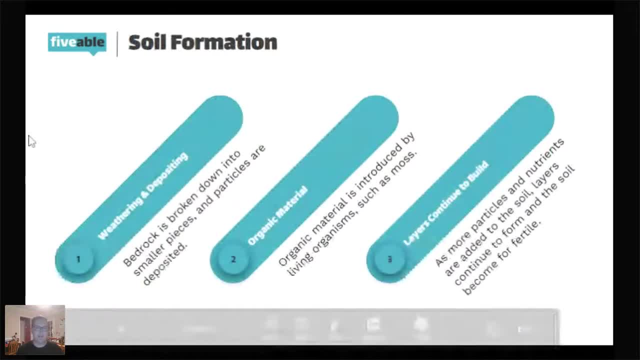 heard of those terms. All right, So soil formation. So there's basically three general steps. Okay, You've never heard of a soil texture triangle. I hadn't either for a long time in the class, but it's really easy, So hopefully you'll get it after this. live stream All. 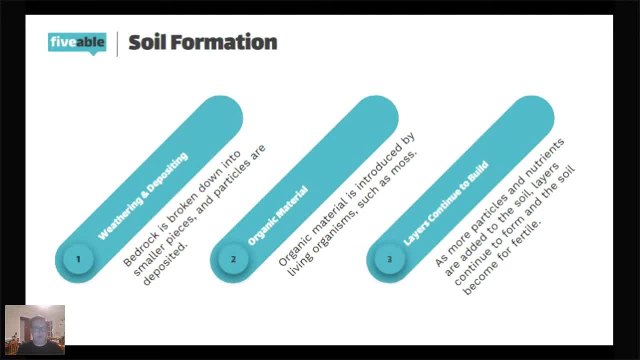 right. So soil formation happens in three main steps. So we have weathering and depositing. organic material layers continue to build. So soil formation happens in three main steps. So we have weathering and depositing, and when you look up here there's a huge meter to show. So those are the main three steps of soil. 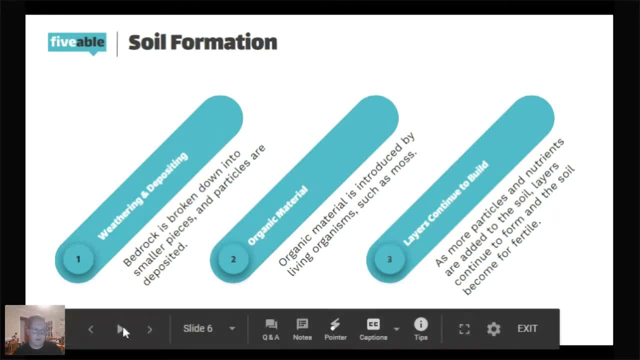 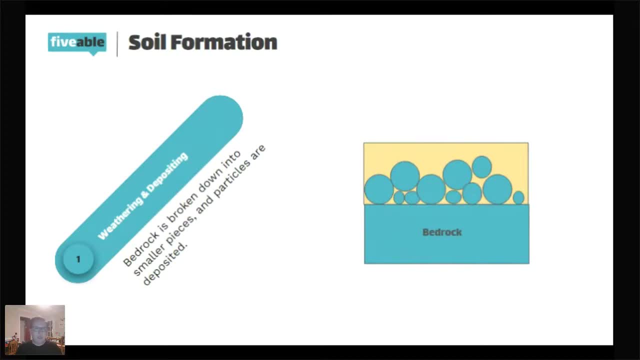 formation. Right, I made some graphics to help better explain this. So first thing that happens is weathering and depositing. Whenever we talk about soil horizons, you sort of kind of see this idea of bedrock at the bottom, and then, as you go up, the particles are going to get smaller and 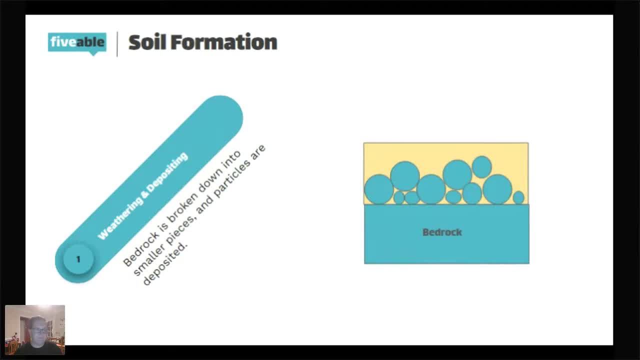 smaller and smaller. So if you look here, look here, get my pointer- These particles are pretty big right now In this video. Okay, So we're going to talk about the field system, so we're weathering stage, but as you get up, you know you have the smaller particles up here, but that's. 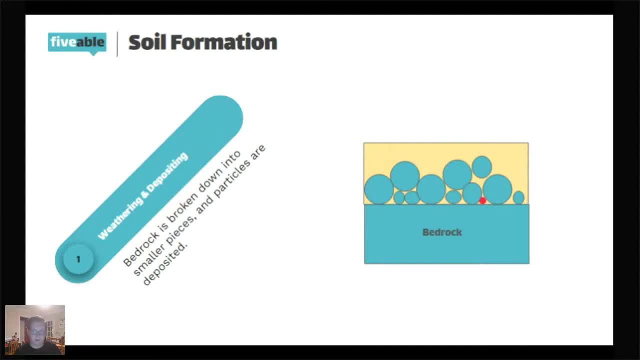 generally what you're going to see closer to the bedrock, or those bigger particles, bigger rocks, um here, um bedrock is broken down into smaller pieces and particles are deposited. so not only do we have the bedrock breaking down into smaller pieces, we have particles that are bringing or 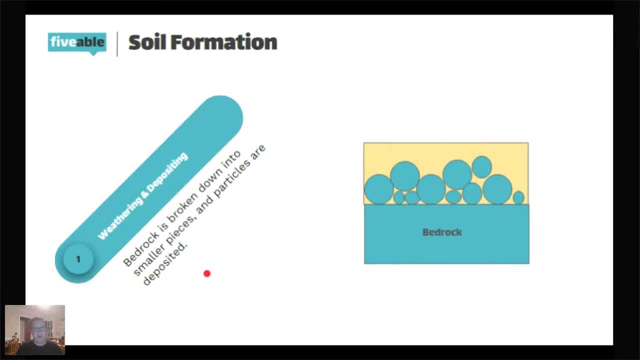 brought in. so maybe a landslide might bring in particles. wind um strong wind can also bring in particles that add on top of it, and that's sort of kind of how we see soil form. it's almost like a layer cake, so you have like one layer um icing cake, if you guys get the relation. 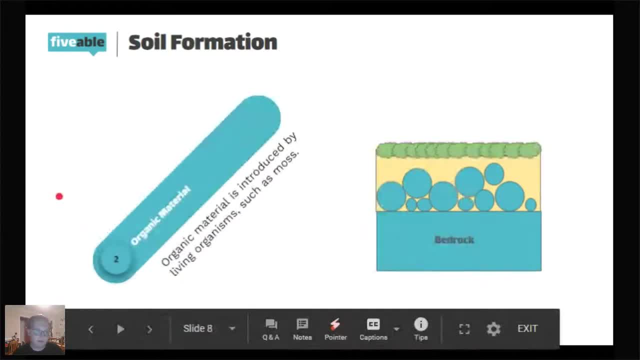 all right, organic material. so now we have a thin layer of soil starting to form here, so now we're going to get things such as moss, um, maybe like small vegetation happening here. we're not going to see a whole bunch of trees or stuff like that, because 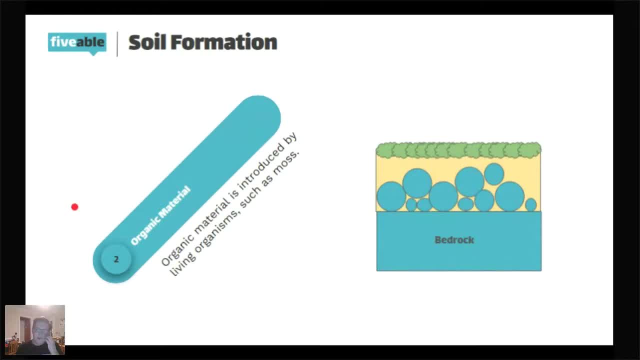 we don't have a lot of space for roots to go um. this moss here is going to help bring in organic materials, so, um, like nitrogen, oxygen, carbon and all those other things will be brought in there as well, as whenever they die, we might see the introduction of bacteria and other organisms. 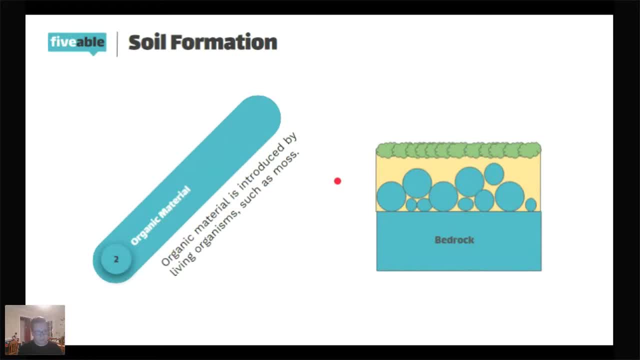 that are going to help break this moss down and add even more nutrients- excuse me, more nutrients- into the soil. um, yeah, so morons, bacteria, all those things are starting to be introduced. so now we're starting to get those layers. so the first step we had rocks being broken down. 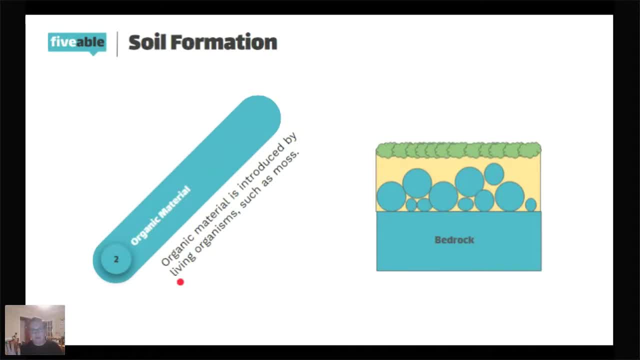 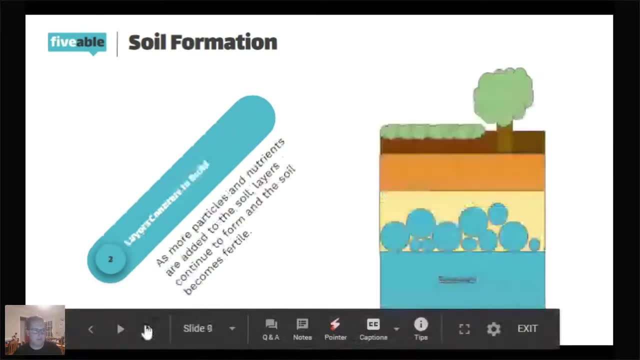 and now we're starting to mix the sediment and rocks with organic material- all right. and then, finally, the layers continue to build. all right. so, again at the bottom here we have a layer of sediment and rocks, and then we're starting to have the bedrock. these rocks, um, are from the bedrock i said before- and then these bigger rocks. 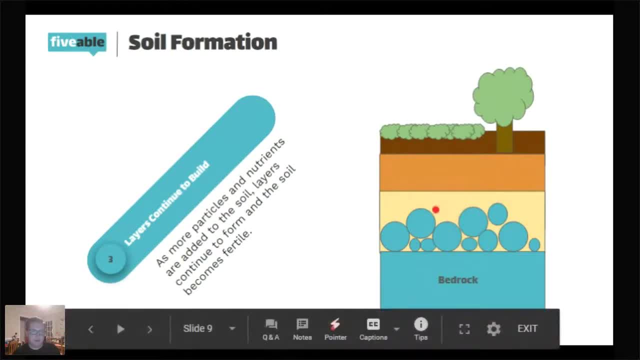 break down a little bit more and as we go up we see that organic, the organic material, increase. so the bedrock and this parent material spot down here isn't going to have much, but as you get up here into this region and this region of the soil, we're going to see more organic matter because 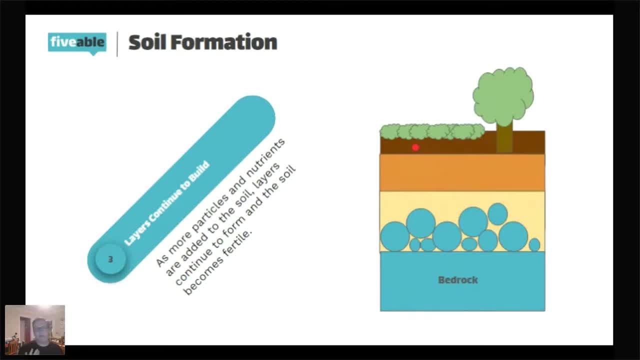 um, we have more biotic factors. um, you might have more organic matter. so we're going to see more organic matter. so we have tree leaves that are dying. they're building into that. um, what else do we have? we have organisms that are starting to move in and we sort of kind of start to see these. 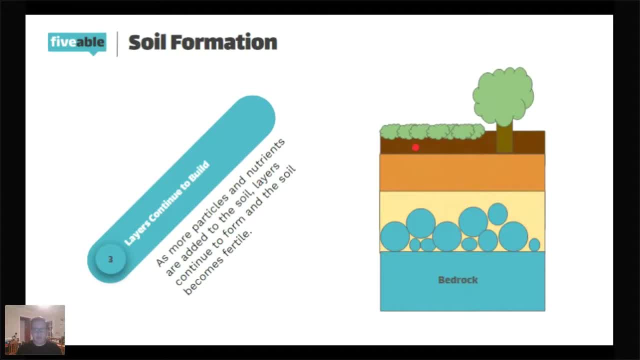 distinct layers, also known as horizon, starting to form, and once we start to get those horizons, then the soil is formed. but always remember, the soil is always changing, so like, um. so all these things are human impact is happening, all this stuff's happening all the same time, so soil is constantly changing. 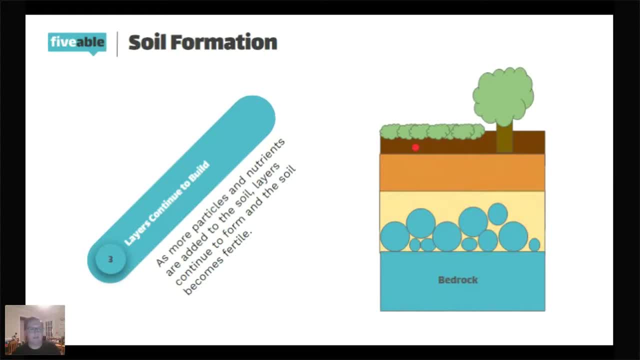 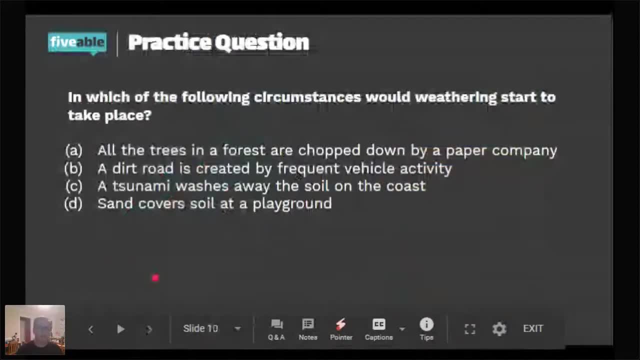 and we'll see how human activity impacts these soil horizons later in the PowerPoint. all right, so here is a practice question. in which of the following circumstances would weathering start to take place? all right, so okay, i won't say that till after um a all the trees in. 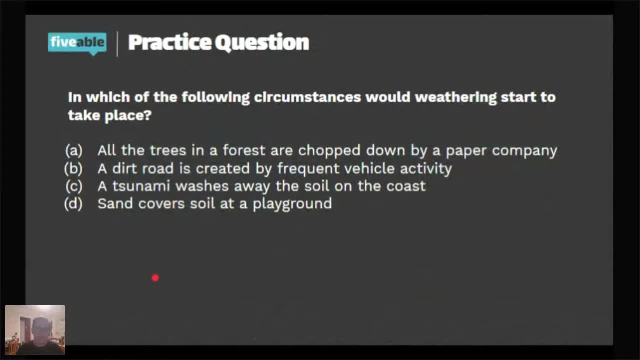 forests are chopped down by a paper company. b. a dirt road is created by frequent vehicle activity. c. a tsunami washes away the soil on the coast, or d sand covers soil at a playground. let me know in the chat which one you think it is. give me a little minute, get some water. 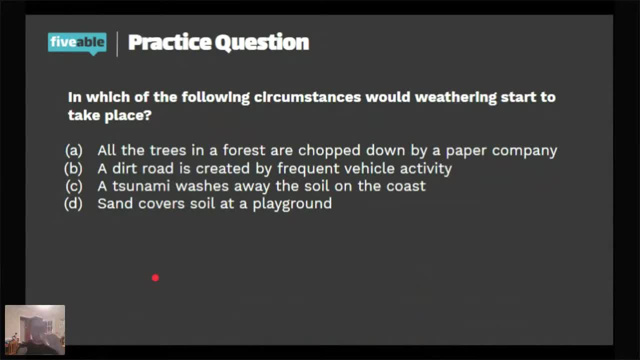 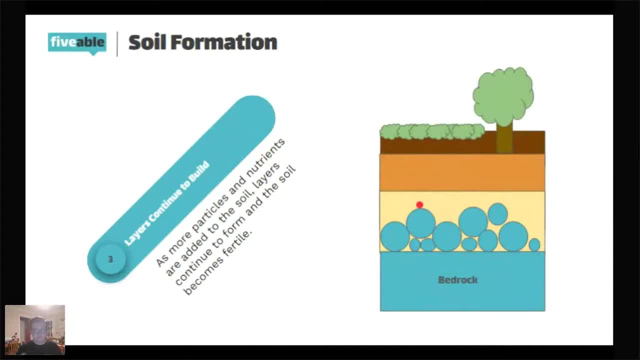 tsunami. but this tsunami is coming in lots of tsunami. but this tsunami is coming in lots of water. water it's stirring up all these particles and it's stirring up all these particles and minerals and all this stuff, minerals, and all this stuff- trees, plants, vegetation- and is washing it. 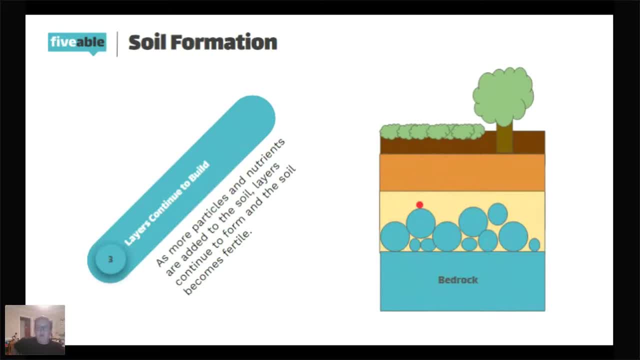 trees, plants, vegetation and is washing it out out, and then we're left with maybe some of, and then we're left with maybe some of the parent material, the parent material, the bedrock- we start this weathering again, the bedrock- we start this weathering again, and then we get our soil restored. 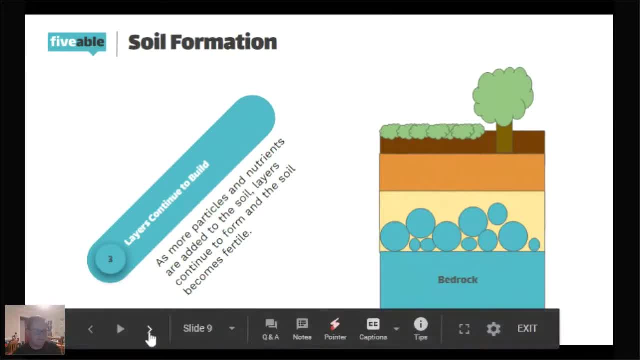 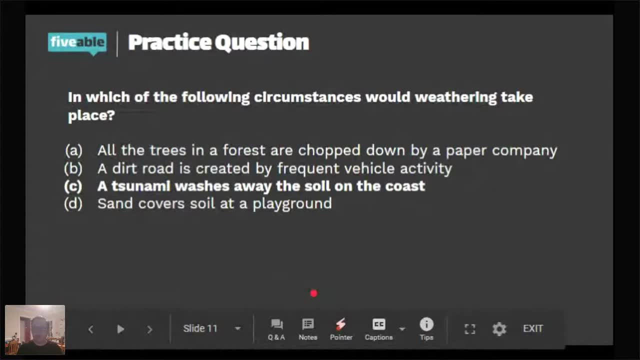 and then we get our soil restored. so it's a never-ending process. so it's a never-ending process essentially, but you can also think about it in. but you can also think about it in another way too like if another way too like if there's a fire and that. 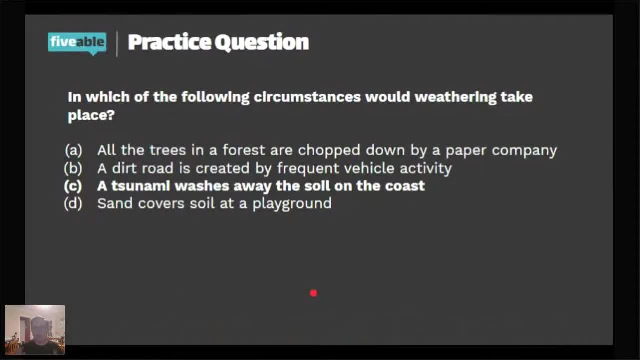 there's a fire and that ruins a lot of the ruins a lot of the um topsoil, then we start to, then we start um topsoil, then we start to, then we start the last step where organic stuff, the last step where organic stuff is moving in. 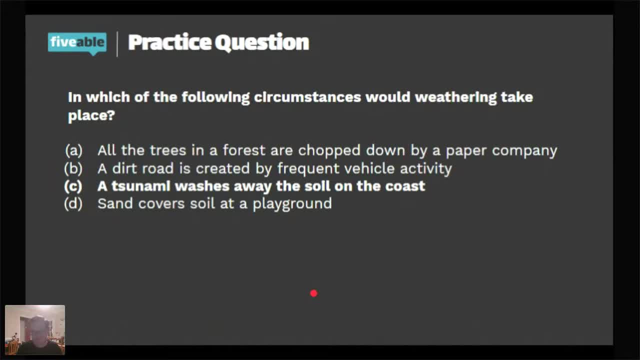 is moving in, replenishing that top soil and getting replenishing that top soil and getting everything rebuilt, everything rebuilt all right, how everybody's feeling good. all right, how everybody's feeling good. up to this point, i'm guessing, so i have. up to this point i'm guessing, so i have no questions. 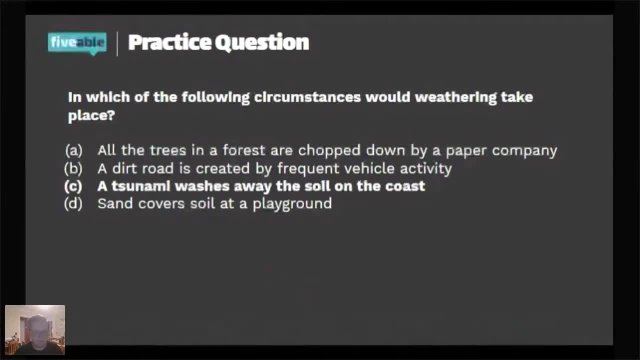 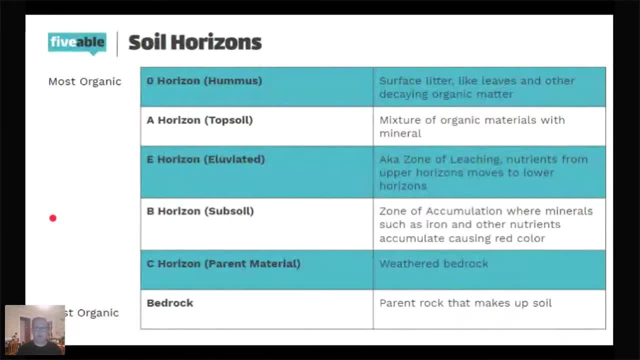 so soil horizons. this is a really important thing, important thing, important thing when it comes to soil. oh, what does when it comes to soil. oh, what does when it comes to soil. oh, what does bedrock look like bedrock, look like bedrock look like? so bedrock is basically like solid rock. 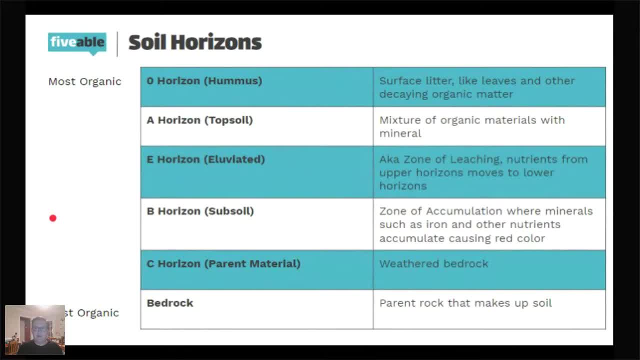 so bedrock is basically like solid rock. so bedrock is basically like solid rock. it's just like one solid piece of rock. it's just like one solid piece of rock. it's just like one solid piece of rock. now the parent material above it is. now the parent material above it is. 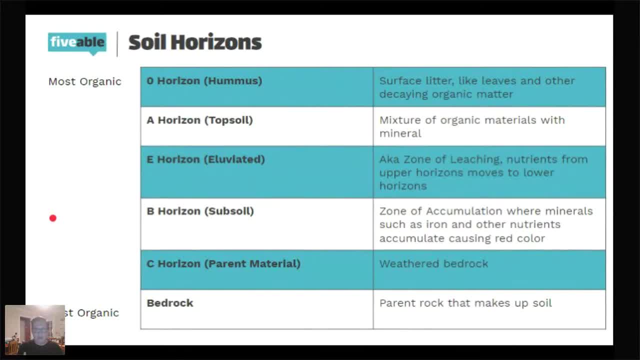 now the parent material above. it is sort of like where the bedrock starts to, sort of like where the bedrock starts to, sort of like where the bedrock starts to crack, crack, crack and make smaller and make smaller and make smaller. all right, so soil horizons um. 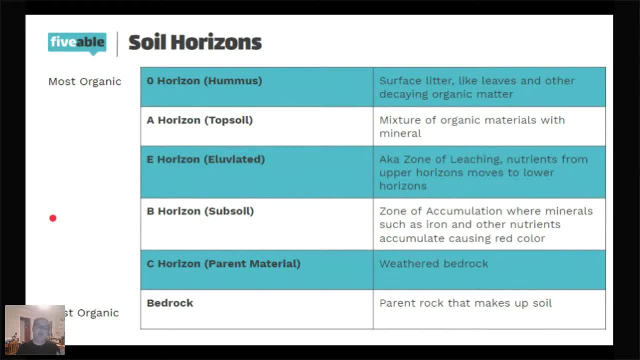 all right. so soil horizons um. all right, so soil horizons um. so the way i like to look at soil horizons, so the way i like to look at soil horizons, so the way i like to look at soil horizons is look at it going um from. 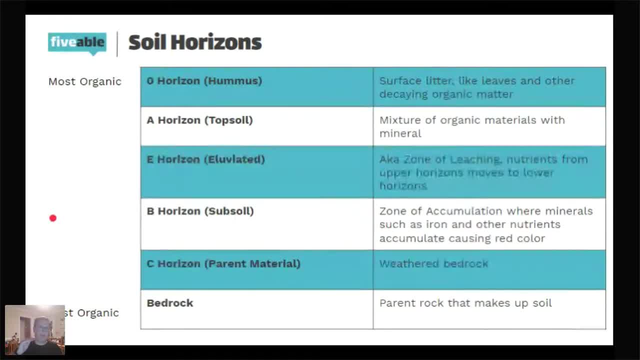 is. look at it going um from is look at it going um from the bottom up and then start to come the bottom up and then start to come the bottom up and then start to come from the top, from the top, from the top down. so if we look bottom we have bedrock. 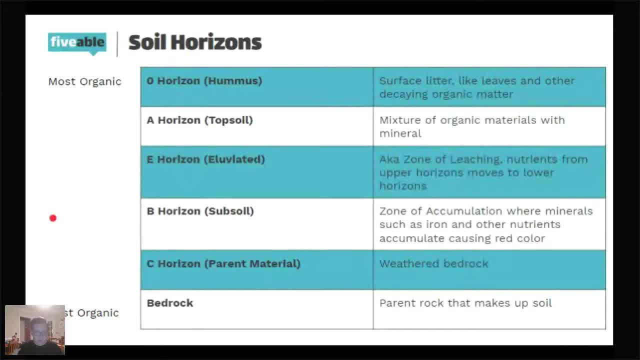 down. so if we look bottom, we have bedrock down. so if we look bottom, we have bedrock, all right, we have bedrock at the bottom, all right, we have bedrock at the bottom, all right, we have bedrock at the bottom and then bedrock. 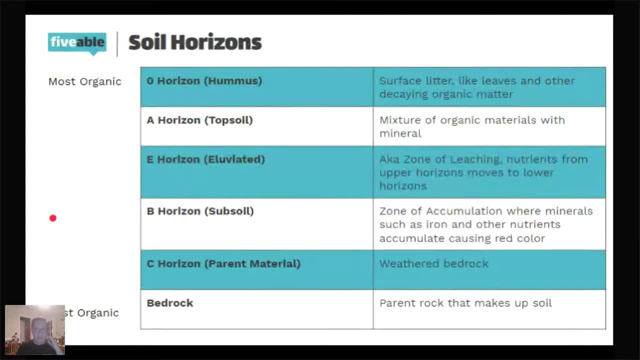 and then bedrock. and then bedrock becomes, becomes weather bedrock, which again is where it starts to crack. we have large chunks of rock and then the horizon. we sort of kind of see even smaller chunks, and as we go up we get smaller. all right, so that's particle size sort of okay. and then we go from the top down, so the top has tons is. 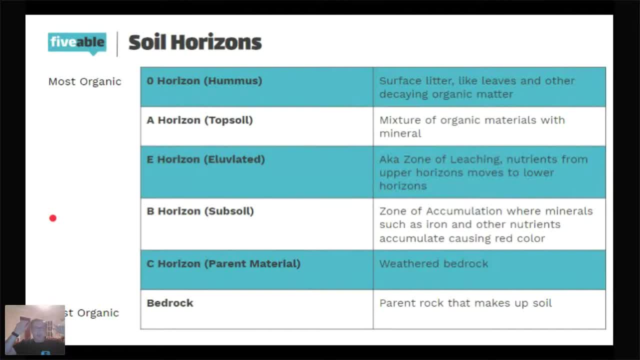 basically like if you guys have ever walked in the woods and there's leaves all over the ground and decaying sticks and the brown, the dark brown stuff, hummus um, that's what this is- leaf litter, decaying organic matters all at the top. then this organic matter starts to sink. 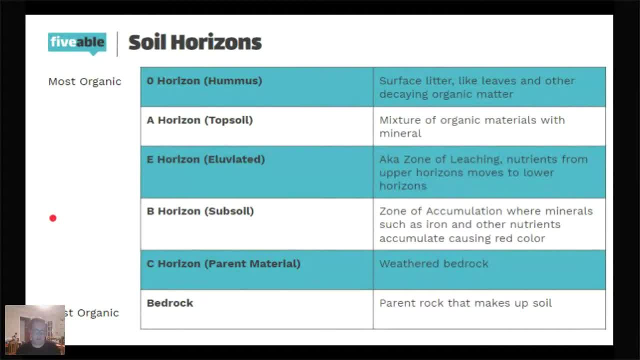 into the soil. so now we're at the a horizon. so at this a horizon we're seeing, like the soil from where we started. this is like the smallest mineral or smallest particles that live here, and now the, now the organic matter is going down into that and then, after the a, 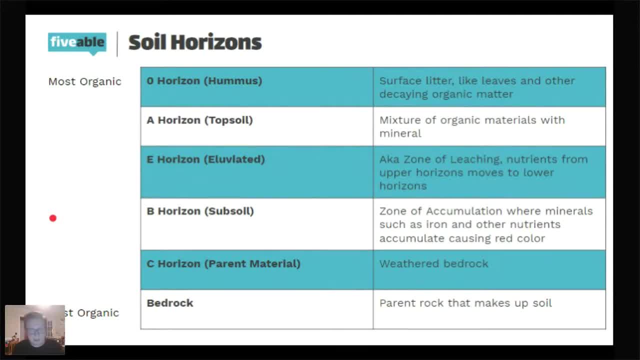 horizon we see the alleviated horizon, um- that might be a new term- um, also known as the zone of leaching. so nutrients from these upper two horizons, the o and a horizon, are moving down into the low horizon. so some of these, like i know, sometimes they won't show the e horizon, but it's pretty important. so work on. 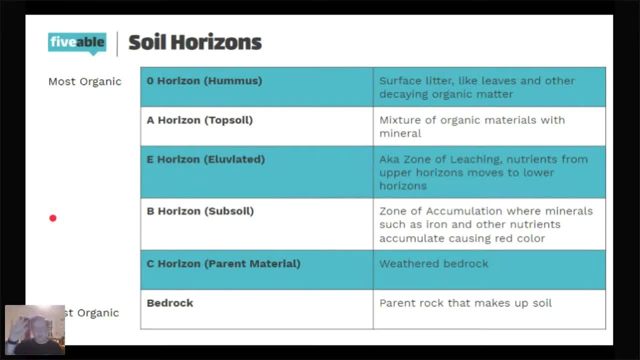 that transition zone between, like the top soil and the organic matter and the subsoil is more mineral rich. all right, so that's what the alleviated horizon is. so we see nutrients, we're moving from the upper to lower, and then we get to the subsoil, which is the zone of 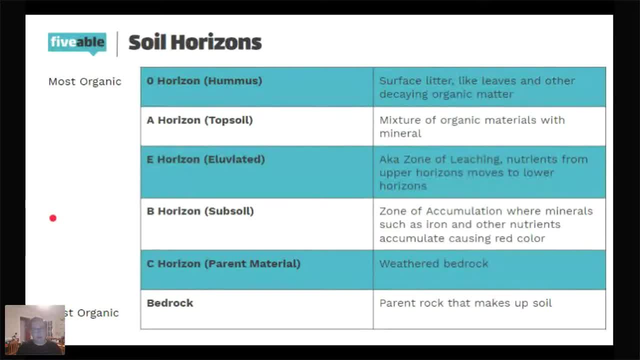 accumulation. so this is where minerals- we have iron accumulating and other nutrients- a lot of times aluminum can accumulate. and then we get to the subsoil, which is the zone of accumulation here and that might create a bright color as we're going down. and then finally, we have 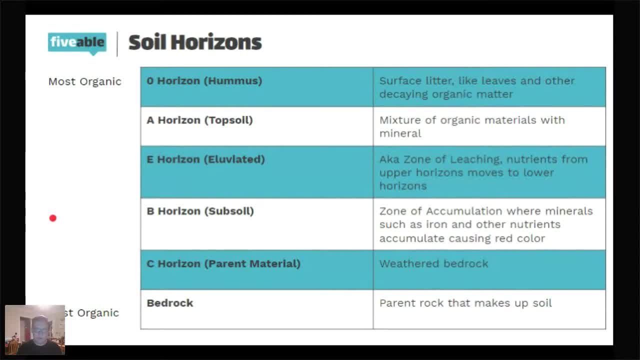 parent um material or the sea horizon, that's weather bedrock. so, um, the bedrock is starting to break up the larger chunks, and then finally we have bedrock which is just rock, like just about solid rock, and then over here to the left we have least organic down here. 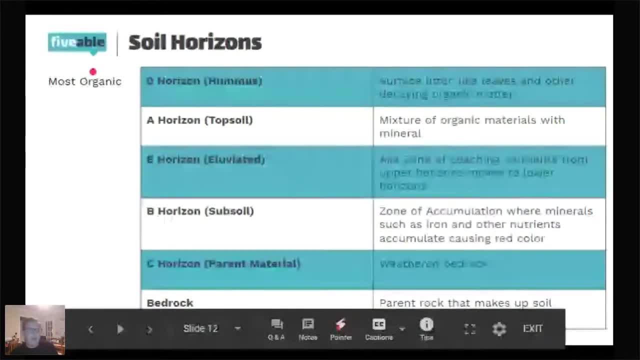 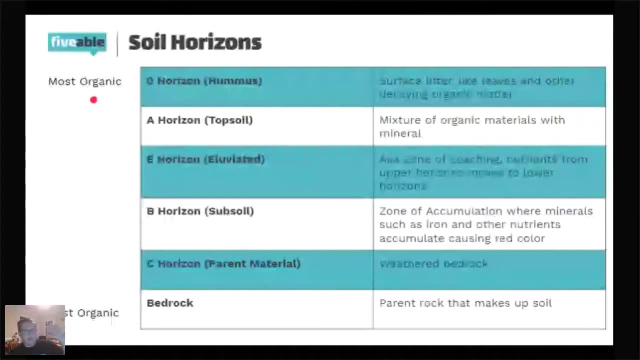 and we have most organic up here. so, as i said before, if you look at it from bottom up and then top down, you start kind of filling the chart. the top is the most organic because we have the hummus, we have the surface litter um bacteria, worms, all the organisms, okay, think the top of the soil. 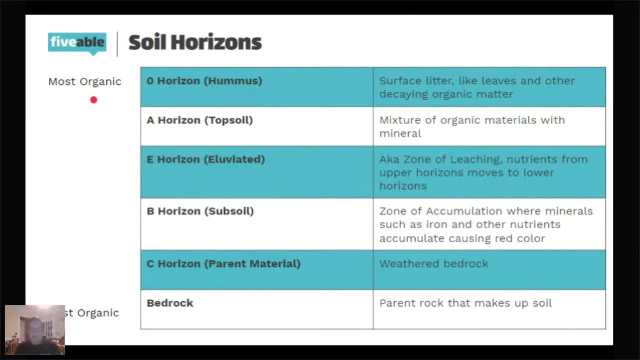 and organisms are living on top of it. so fecal matter, this um, decaying leaves all that stuff. decaying is giving it that organic stuff mean, while down here is the least organic, because for this stuff down here to get any organic stuff we're, we need that stuff from the horizon to go all the way through, all the way down. so and bedrock. 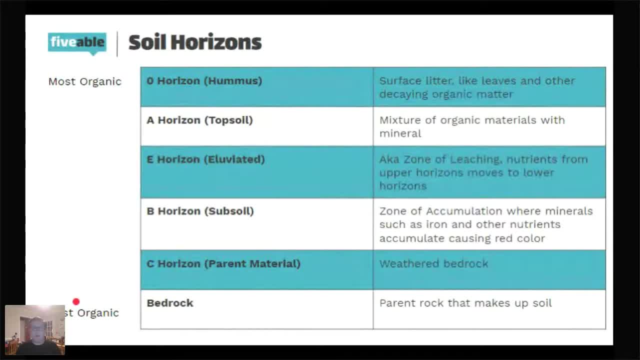 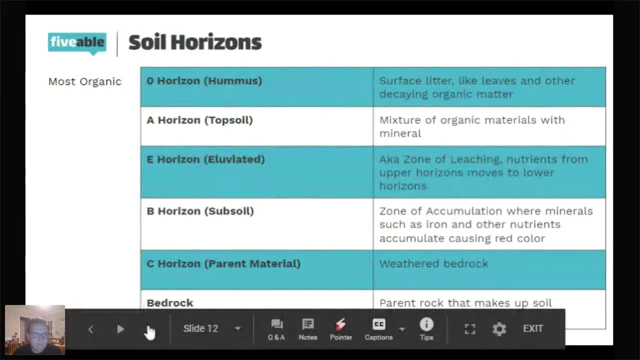 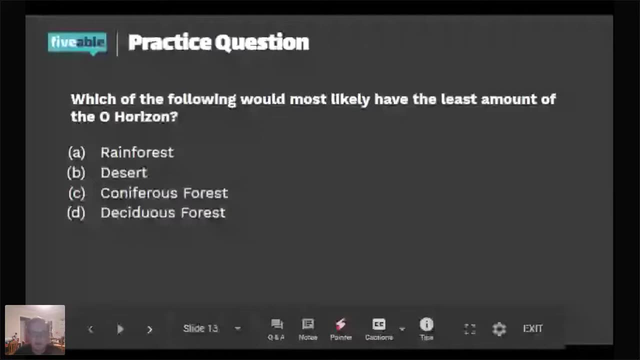 isn't going to take any of that in because it's rock, solid rock. so that is the general trend. so here's another question: which of the following would most likely have the least amount of the home horizon and allow the haah say the least amount? like the thinnest layer, Rainforest, desert, coniferous or deciduous? 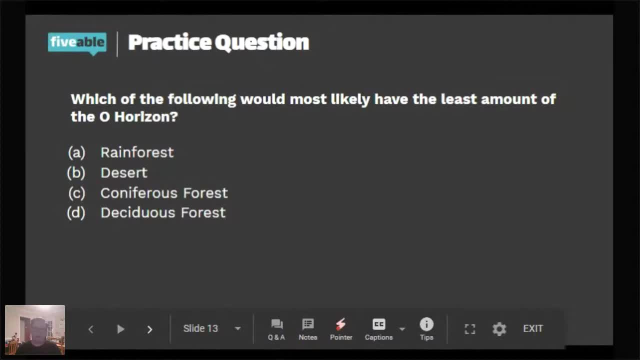 forest. All right, So it would probably be B. So, yes, correct, B, All right. So what is the O horizon made out of? So I'm going to lead you to the right answer. So what's the O horizon made of? mainly, The O horizon is, remember, decaying material. 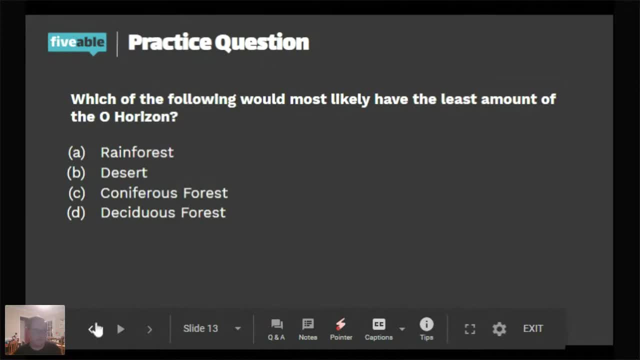 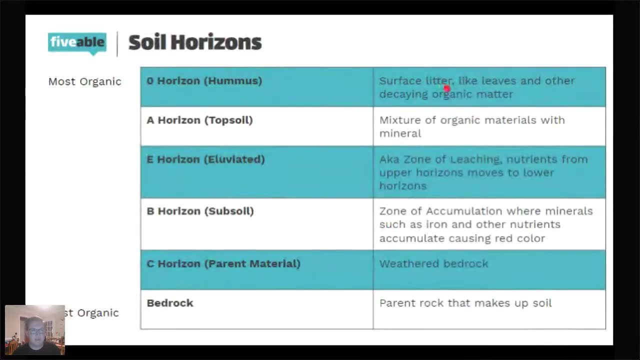 Okay. so the O horizon. Okay, I'll go back, It's all right. So remember this O horizon. here is the surface litter like leaves and decaying organic matter. So if you start trying to think about a desert, usually I have sand, sand, stuff like that. 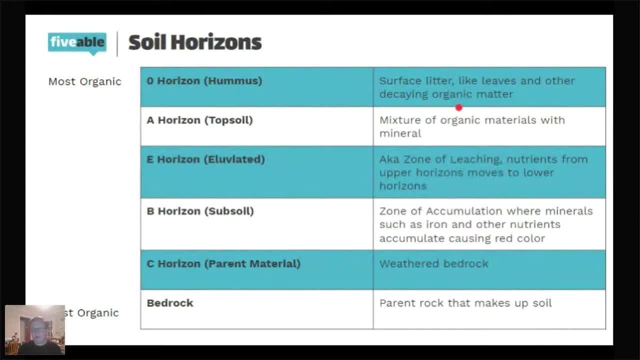 So and we're not saying much stuff decay Like, if you compare, woods has a lot right, because we have decaying leaves, sticks, animals, But in the desert biome it's mainly desolate. You guys, you guys see where I'm coming from. 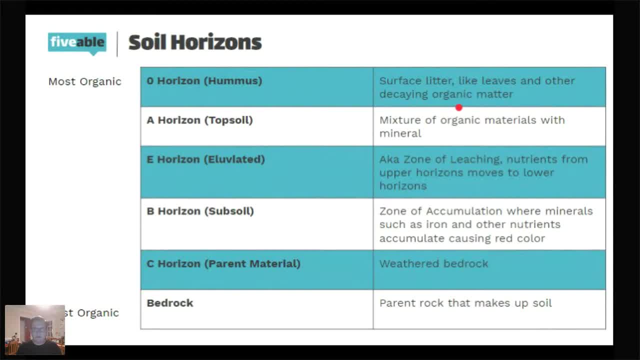 No, the desert doesn't have a lot of dead organic matter. The forest? I might have missaid that. The forest has a lot of dead organic matter. The desert does not. That's why it has no oh horizon. The desert would probably be the sea horizon. 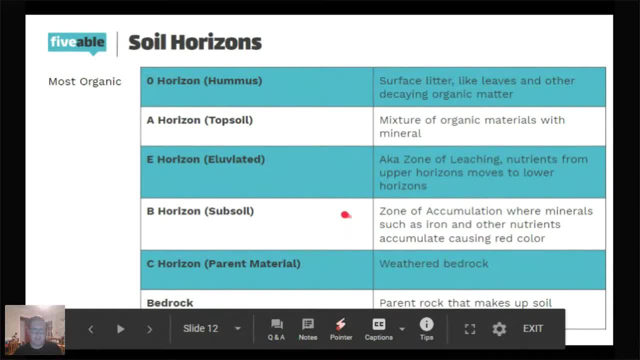 The sea horizon and maybe the B horizon, because we still have maybe some minerals like iron and stuff getting down in there And we're going to talk about that later in the later in the PowerPoint as well, when we talk about different soil horizons and biomes. 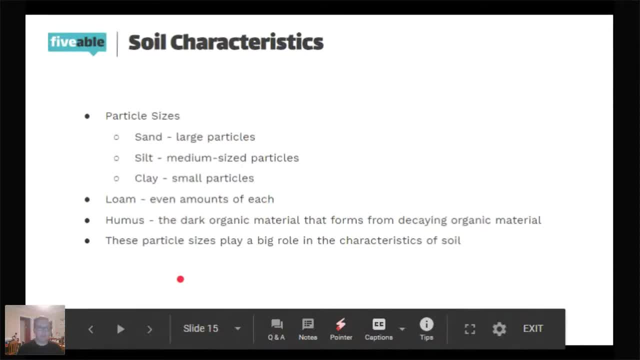 All right, So now on the soil characteristics. So the first type of characteristics are usually categorized by three things, or three, Okay. They're characterized by particle size. We have three main particle sizes. We have sand, which is the larger particles. 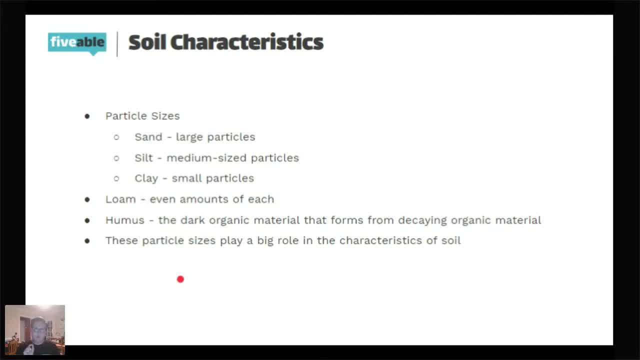 Silt, which are more medium sized particles, And then clay, which are the small particles. Loam is even amounts of each. So when we get to the soil, texture triangles we're going to have. we're going to have like percentages, like percent clay, percent silt, percent sand. 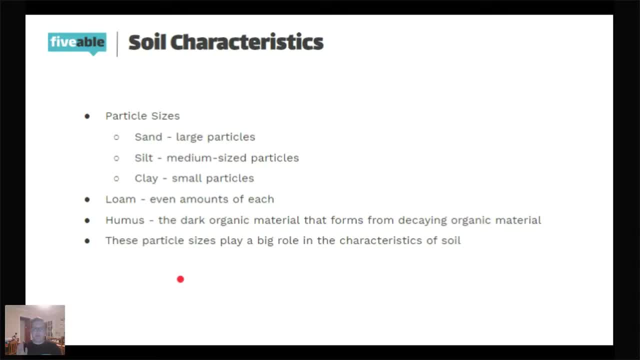 And so loam. whenever it says loam on that, that means even, Even amounts of each, So you might have 10% sand, 10% silt or no, sorry, like 30% sand, 30% silt and 30% clay. 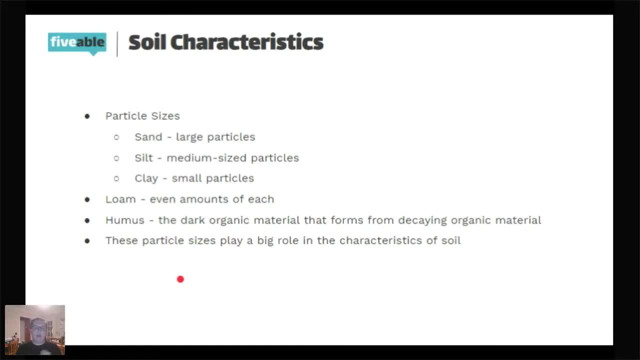 Or just about even amounts Hummus. I didn't define that earlier, but that's a dark organic matter that forms when from decaying organic material. So that'd be again your O horizon that we were talking about earlier. And these particles do play a big role in the characteristics of soil, as we will see on the next slide. 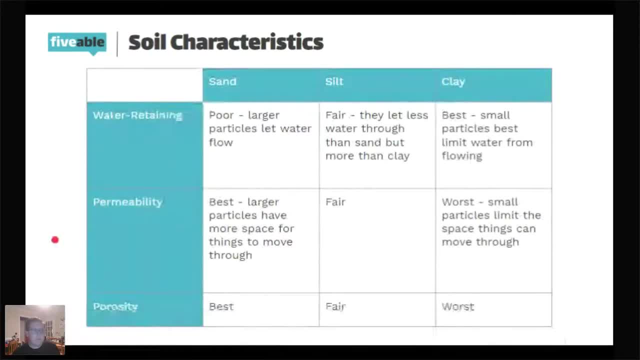 All right, so here are a few characteristics from the CED. Okay so, trying to find a way. Okay so, water retaining sand is very poor at retaining sand. If you think about it this way: say, you have a sheet and you put a whole bunch of big like glass circles on it. 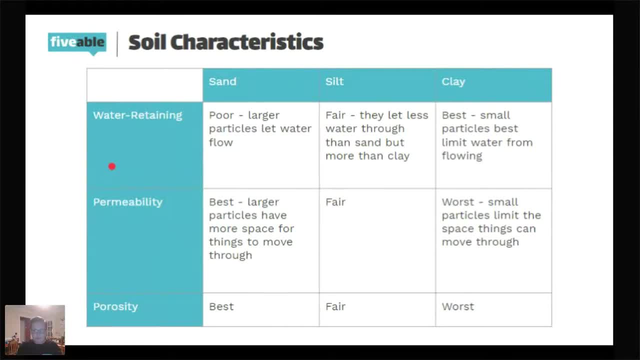 There's going to be more space to get through. if you like, push them off If you put them all together, think about it. But anyways, the bigger particles. when they are crammed together, there's more space between them. 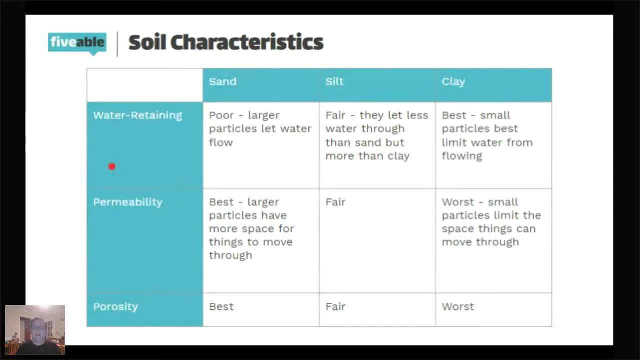 So that's going to allow water to go through. Therefore, the sand soil with a lot of sand in it is going to let water flow through faster And then silt. it lets in less water than sand, but more water than clay because it's smaller and can fit together better. 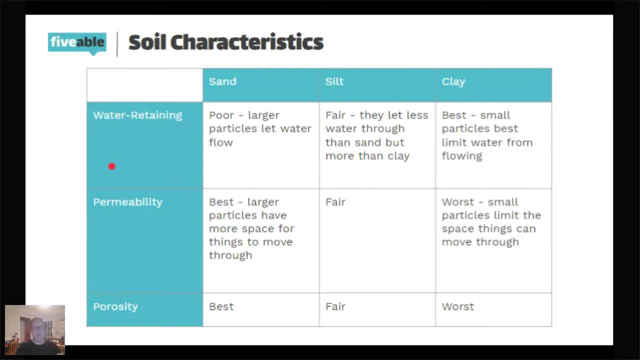 And then clay, finally, is the best Because the smaller particles best limit water from flowing. So if you have soil with a lot of clay, that might be the best for retaining water. Like, say, you have a pond and you're like: is it going to make a pond here? 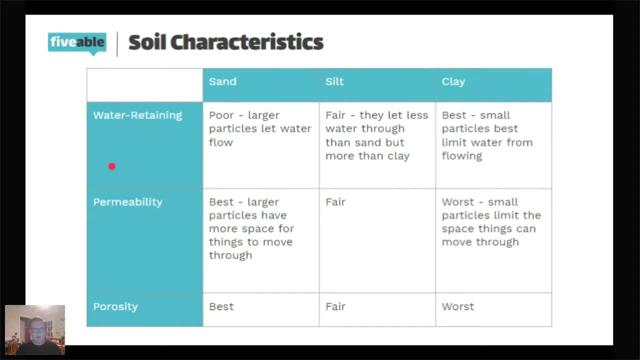 Well, probably wouldn't be good to make a pond on the beach because A you probably have waves, But also the soil there is very sandy. It is sand And any water that you put on like in a 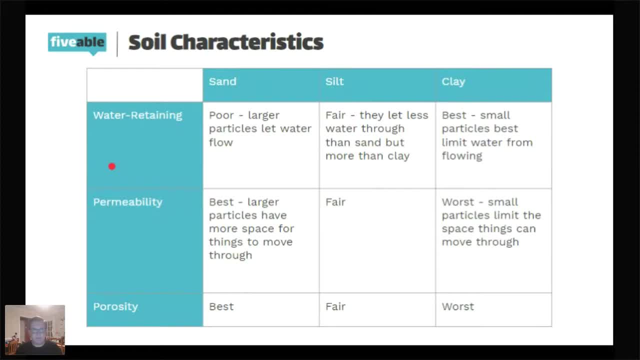 dugout thing of sand is just going to go right through. So yeah, But also, if you think about it, clay bowls that they make hold water, So that's water retaining Permeability. This one kind of follows the same thing. 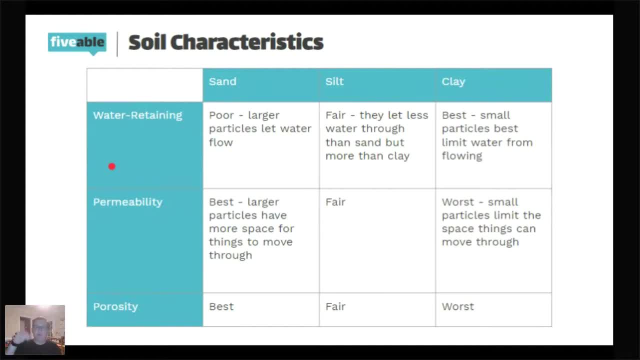 Permeability is the ability of water or air to get into the soil. Again, sand is going to be the best for this. It has more room to get through, It can move through, And then silt is fair. Again, it lets more in than clay, but less in than sand. 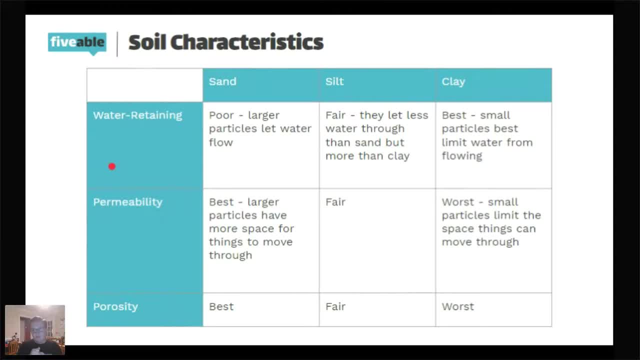 Excuse me. And then clay is the worst because the small particles together are. They're not going to let anything through the small particles. And then porosity And these all sort of kind of follow the same thing. So permeability is the ability of air to go through. 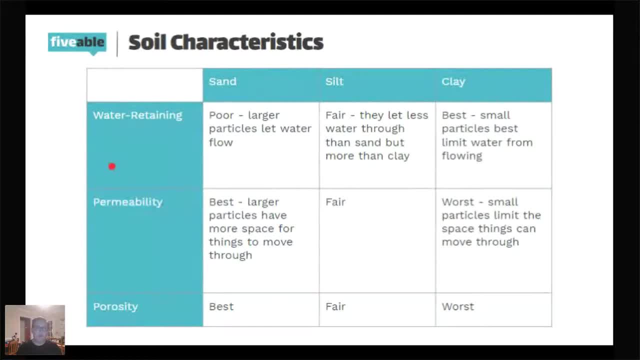 Porosity is the ability to hold air. Hold air, Hold water. Again, sand is the best, More room, Silt Fair And clay is the worst. Does that make sense to you guys? Make sense a little bit, Hopefully. 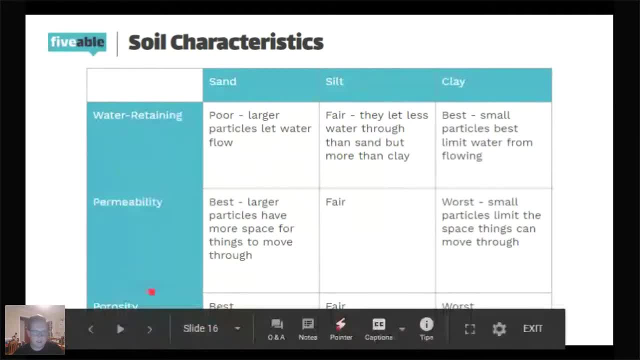 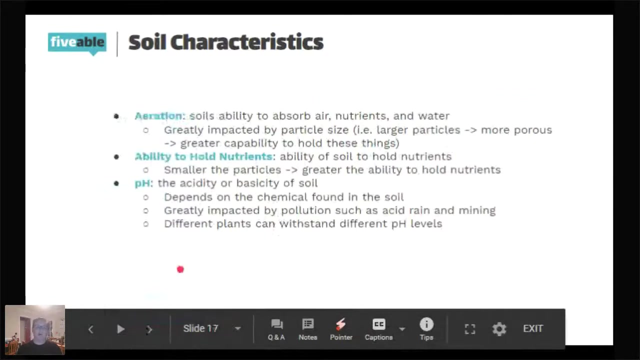 Yes, All right, Sounds good. All right On to the next. Now it's porosity. Think poor, Able to hold air. It was: Yeah, Yeah, All right. So there are also some other soil characteristics that might less depend on particles. 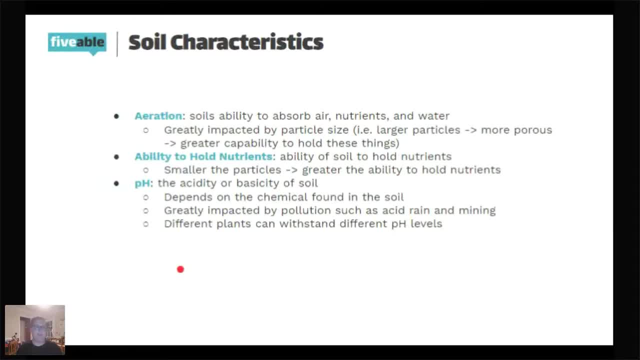 So aeration, So the soil's ability to absorb air and nutrients and water. Again, this goes Okay. So, based on what we learned in the last, In the last, On the last slide, Which of the following particles do you think would be best for aeration? 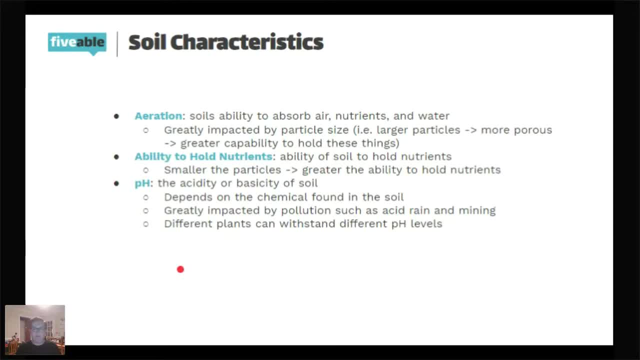 In the chat. Which of the Sand- Yes, The size particle that would be best for aeration, Yes, would be sand Sand. Now I want to clear something up Because, like, if you have sandy soil, it's not all sand. 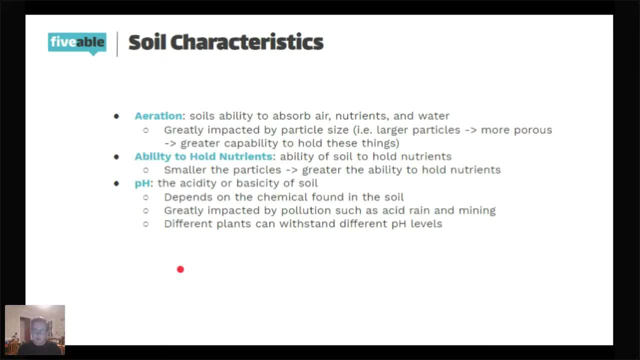 And remember, there's also the parent material And there's also organic nutrients coming in. Okay, It's sort of the same. Okay, Soil is very- Yeah, Basically dirt, But there's a lot more to it. It's like soil is dirt but 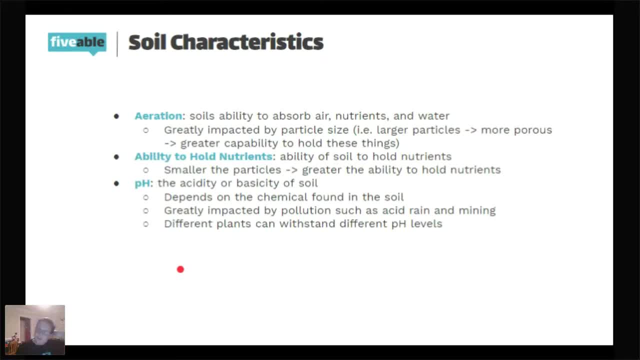 I don't know. That's a tricky question, But yeah, they're basically the same thing, Like if you go outside in the grass and start digging, that's soil. Yeah, Soil is. Soil is a broad term. yes, because there's a lot of different characteristics that go into it. 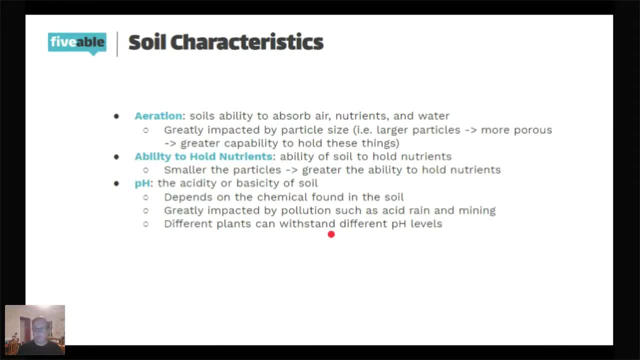 pH aeration what the soil is made out of. Like the soil in grasslands is different than soil in the desert. Coastal sand is different than grassland sand. So yeah, soil is a broad term, All right, So does that clear everything up? 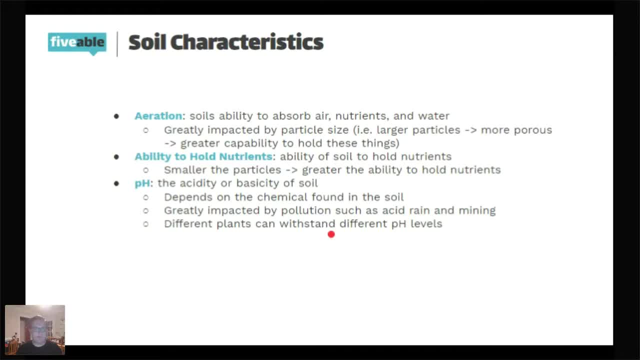 I'm glad you guys are asking questions. All right On to ability to hold nutrients. Oh, also aeration, yeah, Larger particles like sand, more porous, greater capacity to hold these things. nutrients, water, air, All right. 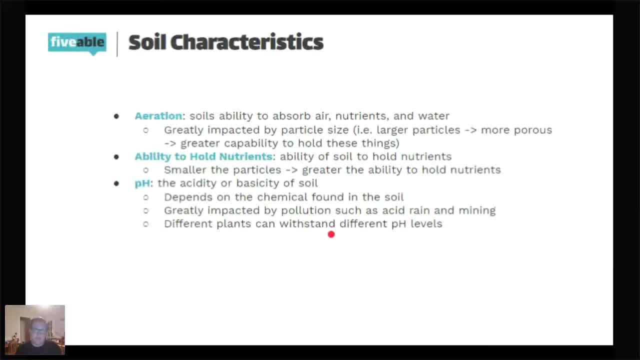 So next we have the ability of soil to hold nutrients. So think, Because, like whenever I first read that, I thought I had something wrong. But no smaller particles have greater ability to hold nutrients, So yeah, 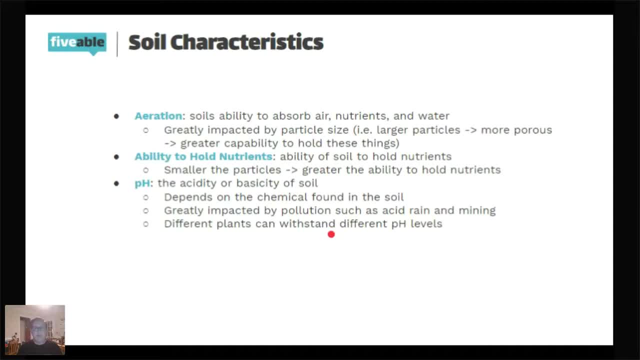 That just goes with what we've been saying. Really, the ability to hold anything is based on smaller particles, But then aeration, the ability to absorb, is the opposite. We want larger particles so it can get in and smaller particles to hold it in. 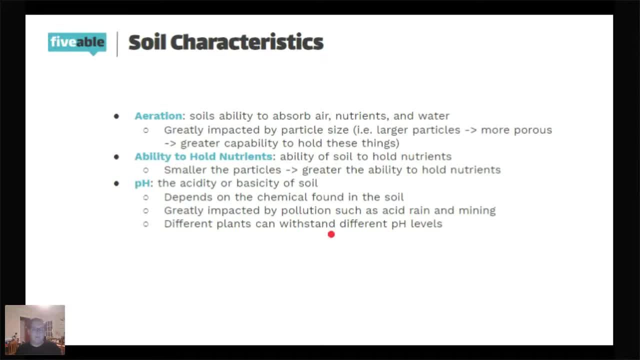 And then finally, pH is a chemical property of soil and greatly impacts the plants that grow in it. So we have, So it's basically the acidity or base system. So the acidity of soil depends on chemicals found in soil greatly impacted by pollution such as acid rain and mining, and different plants can withstand different pH levels. 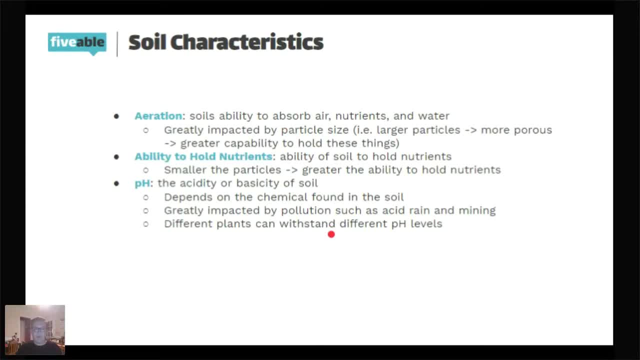 So the acidity of one soil might be good for certain plants and some, and low or other acidities might be good for other plants. And one thing: whenever your pH gets too low and very acidic in soil. So the acidity of one soil might be good for certain plants and some, and low or other acidities might be good for other plants. 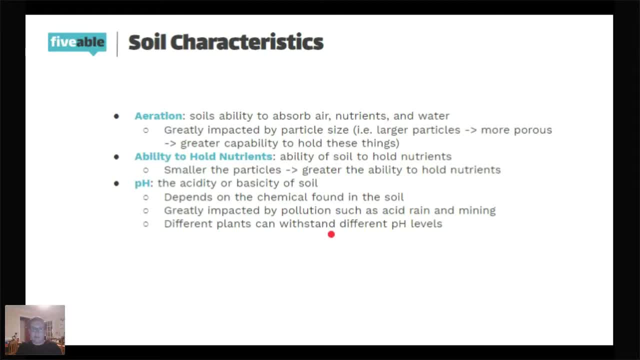 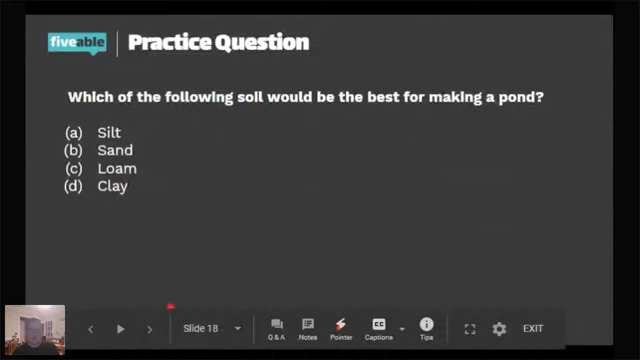 You start to see acidic resistant weeds start to come up. So that's sort of kind of how pH plays an effect, Definitely the type of plants that are growing there. Okay, So clay, Okay So I know clay, you think like the art clay, but sort of kind of think of it as like a particle, like a tiny particle. 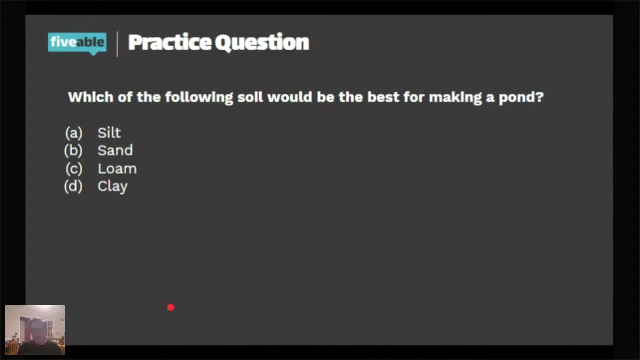 that's really really, really, really small, like- oh, i think it's like 2.5 nanometers, really really small, like sand, silt and clay. they're mixed in with other stuff in the soil but if you have a lot of clay, a lot of the small particles coming together, then it's holding stuff in. 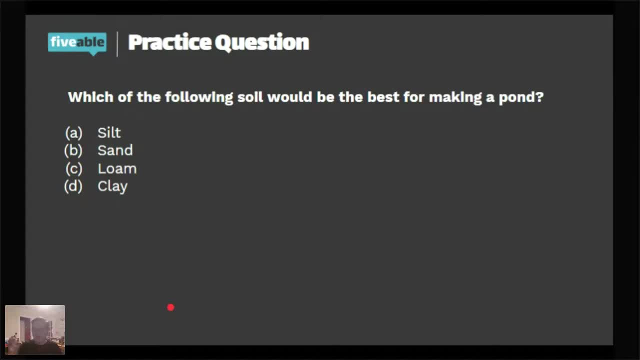 the same with sand. it's not all sand, but it might be sandy. like with everything else mixed in the organic materials and the parent materials, there's a lot of sand mixed in. does that make sense? i hope that makes sense because that's what i thought as well, um. 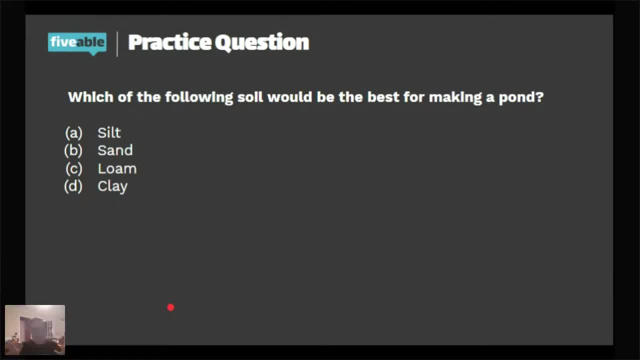 like a clay, like a piece of clay that you'd use and i'm like it doesn't make sense, but it, like everything about it, does the particles. okay, makes sense, all right. so which of the following soil would be best for making a pond, a silt b? 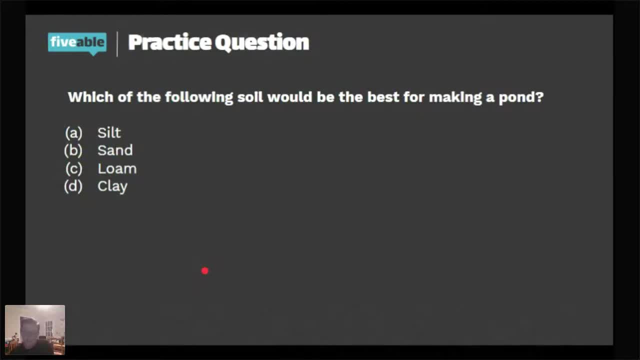 a silt, b sand, c loam or d clay- okay, not which of the following soil- i'm going to correct myself- soil that has the most of which. so, if you're looking for soil to make a pond, what do you want? which of these would you want most? which of the particles would you want most? sand? 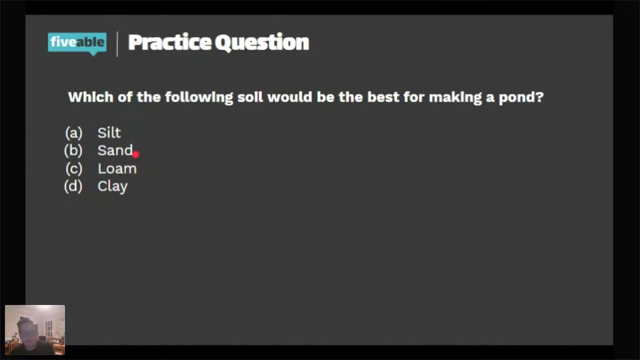 yeah, it would be clay. you'd want a lot of clay. okay, not which of the following soil- i'm going to correct myself. clay, um. you'd also want sand as well. i guess it depends on the pond you're making. but clay, yeah, because you want, you want that water to be held in, um, but also remember, you can't have sand in there. 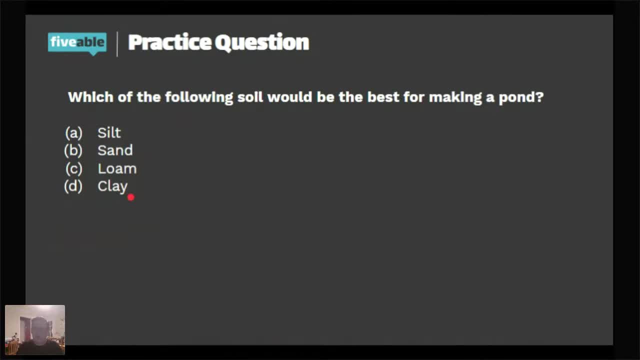 because it's really particles. so you want, you just want- more clay particles. i just really want to stress that because that can be very confusing. all right, all right, which soil horizon will would permeability most likely affect? uh, hold on, i'm going to put this in the chat. 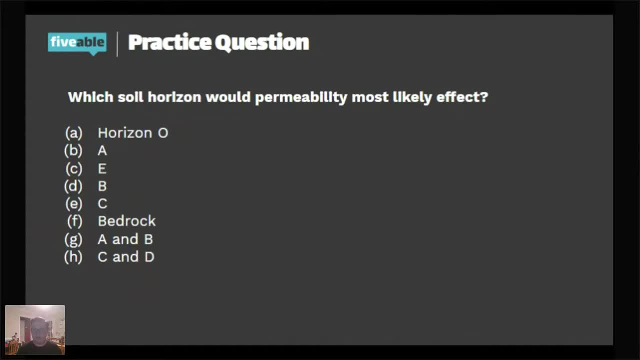 this, um, what i just put in the chat. there is the link to this powerpoint so you guys can look at it. yes, g, a and b. yes, Yeah, I thought that would help, So you guys can look back. Actually, it's H. 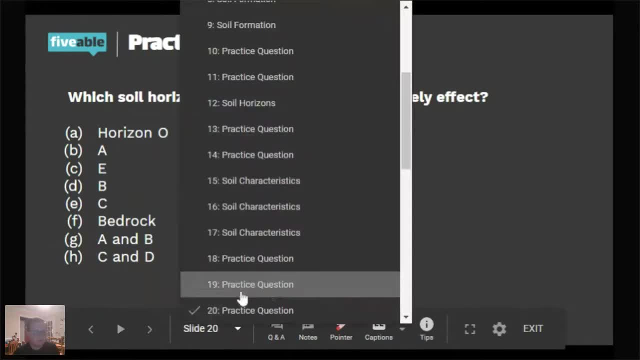 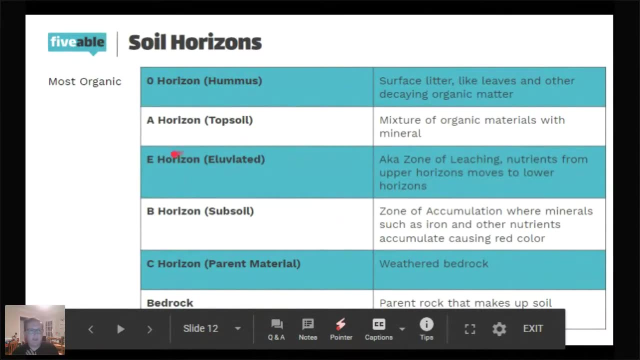 Let me go back to the soil horizon thing. All right, So we said so. I said it was E and B, All right. So remember, E and B is where the nutrients are going through the soil, the zone of leaching. So if the soil is very porous, 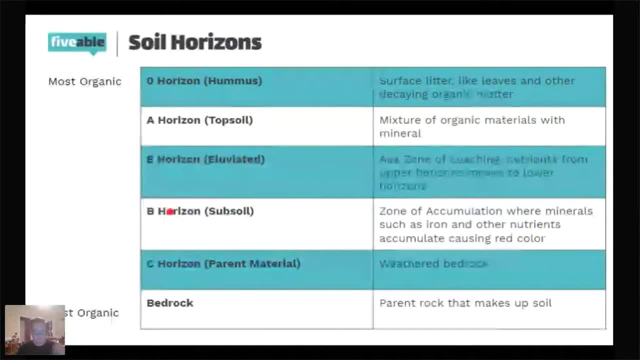 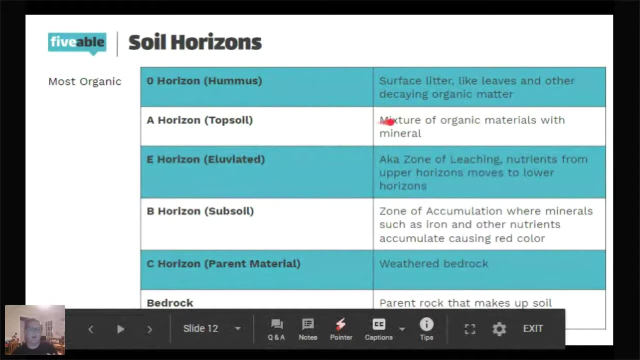 then it can. then the nutrients can move down And also, with the B horizon zone of accumulation, those nutrients coming down. But I must admit that it really could affect all of these things, because this topsoil is going to have different stuff based on porosity or permeability. 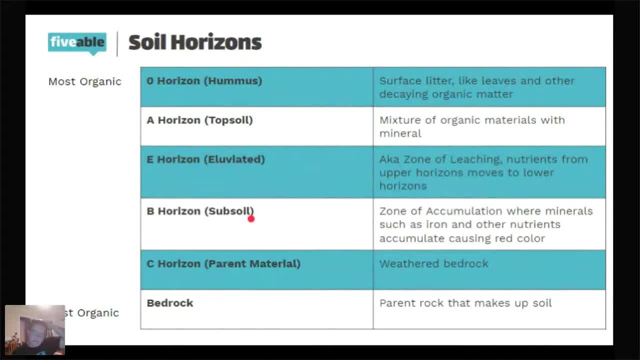 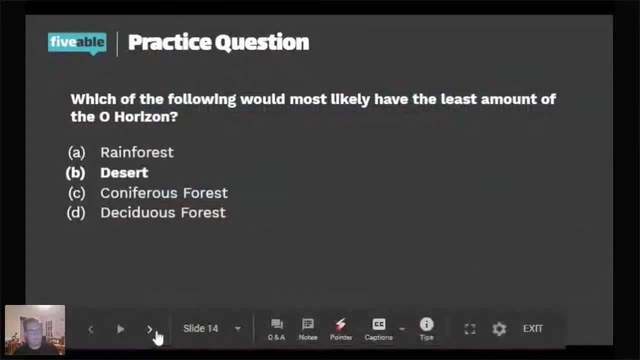 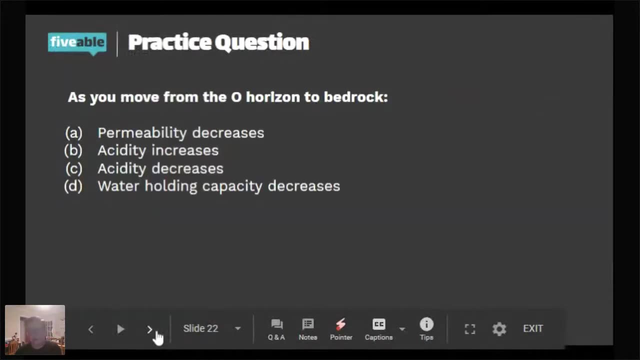 But these E and B are going to be most affected by that. See how far these nutrients can get down. Does that make sense? Yes, All right Sounds good, And if not, always be sure to let me know, because I will be sure to answer. All right, So as you move from the O horizon to bedrock, 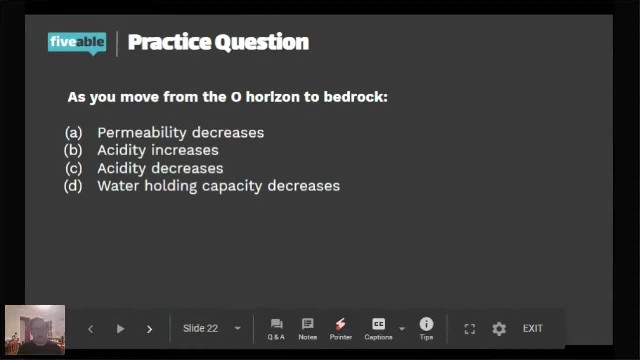 A permeability decreases, B acidity increases, C acidity decreases and D water capacity decreases. Yes, A Yes, Because remember O horizon. we're going to have O horizon. stuff can come through, As you know if you've ever watered a. 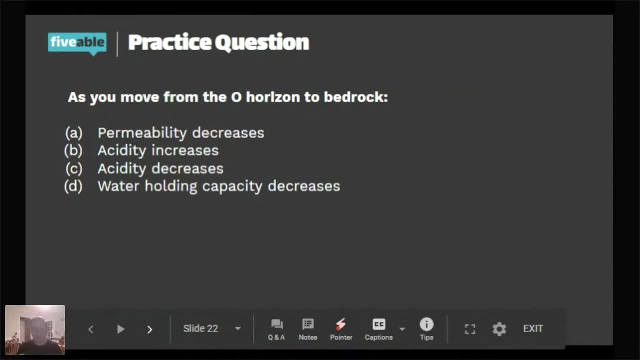 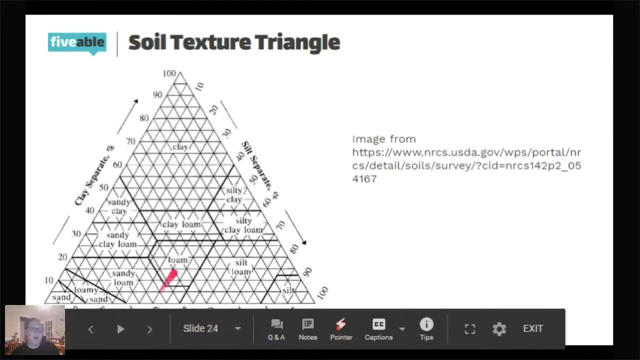 plant water can get through, However a bedrock- it's solid rock. Nothing's really going to get through that unless it seeps through a long way. All right, Permeability decreases, All right. So this is the clay triangle. If you guys did the PowerPoint. 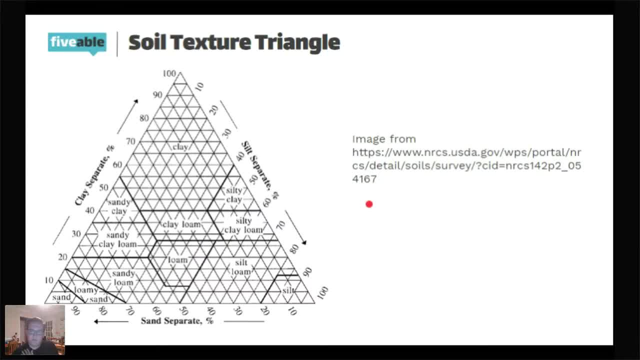 did it work for you guys? whenever you pulled it up, Have you pulled it up? Because if it did, if you guys want to go to this link, there's a better picture of it, if you need to, if it's blurry, If you can see that, fine, then that's great, But if not, you can visit that link. 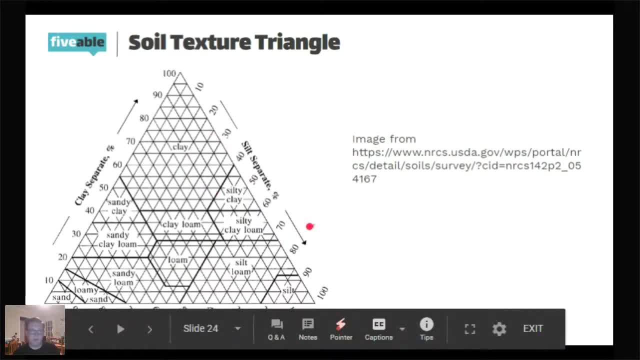 And this is where I got the image from. It's from the USDA, US Department of Agriculture, And some some. if you Google it, you can also find colored images which help. But you know, if you want to go to the next slide, All right. Then on to the next slide, All right. 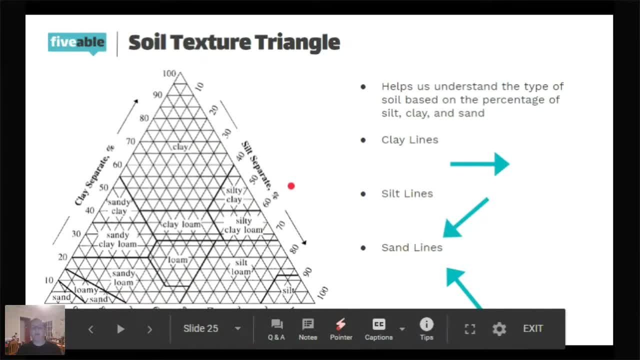 So this soil texture triangle helps us classify soil based on the percentages of silt, clay and sand. So, as you can see we have, if we look over to the side here we have clay separate percent And that just means the percentage of clay, The silt separate by percent And the sands separate. 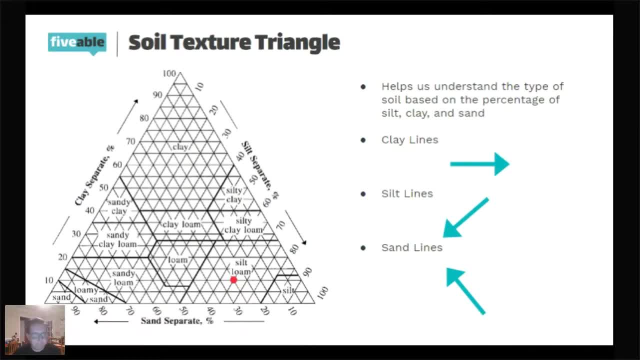 by 25 percent. All right, That's good. Okay, I wasn't sure if the link worked, But that's good, All right. So these are the clay lines that go straight across the triangle. So if it says 70 percent clay, you're going to the 70 percent line and you're going straight across. 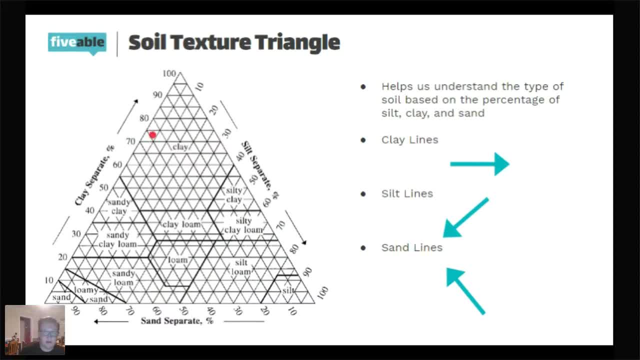 It's not really straight the way I'm moving my mouse, But I hope you guys get the picture. Silt lines are going. it might the line might be going. look like it's going this way, the way the arrow's pointing. But 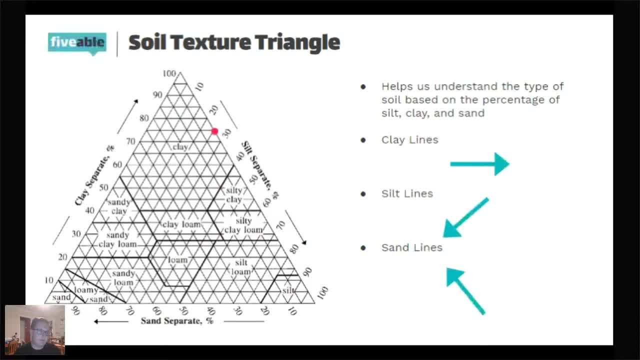 the silt lines are going this way down. If you look at the numbers, the way the numbers are going, the silt lines are going, silt lines are going down And then the sand lines are going up this way, This way. So 50 percent would be here Going that way. Yes, This is also part of the CED Soil texture triangle. Yes, 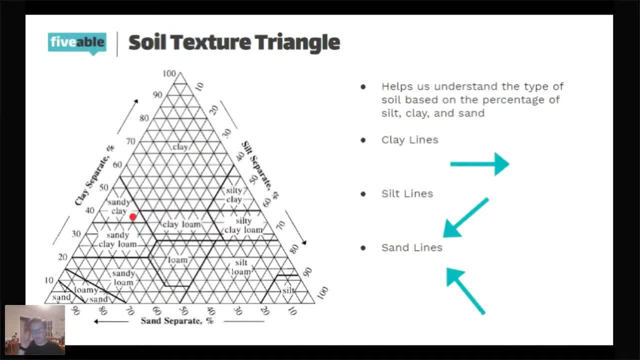 Yes, This is also part of the CED Soil texture triangle. Yes, Yes, But it's not that complicated, I promise It's not that difficult. It's not that complicated, I promise It's not that difficult. The CD is the course exam description. So if you type in your search bar AP environmental course exam description, There's a long PDF with everything you have to learn. 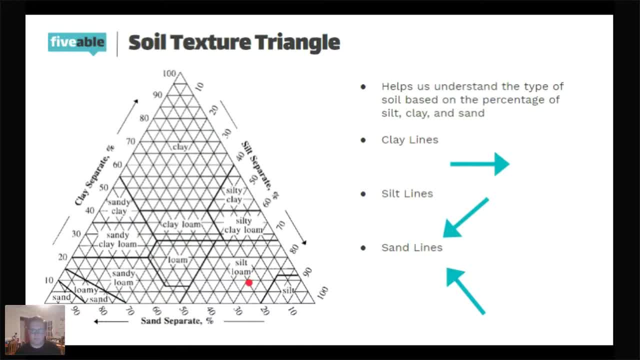 You can't fix it now, but you can work with the CED to get it to work. So yeah, This is. This is part of the soil unit. This is part of the soil unit. So yeah, This is part of the soil unit. 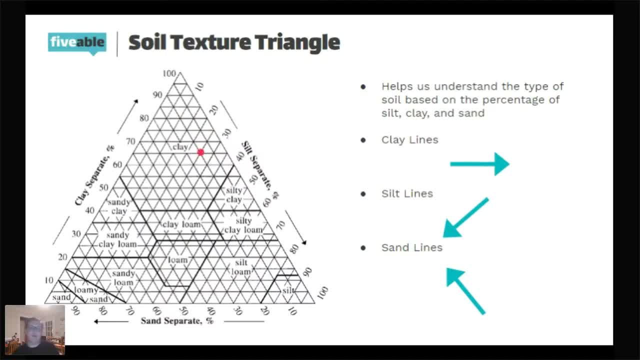 Like this: This is part of the soil unit that they have in there, or soil topics they have all right. so basically they're going to ask you like: okay, so there's 60 clay, 30 silt and 10 sand. so in that case, you're just going to um. 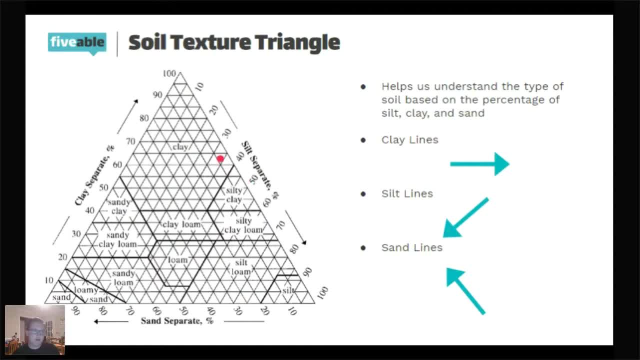 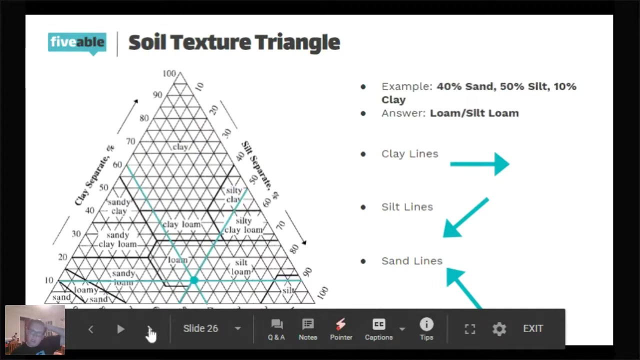 like if this was on paper right now i just draw over. i think, yeah, 30 silt, i'd make that line bold. the 60 clay, make that real bold. or the sorry, sorry, sorry, 60 clay going this way and 10 sand going up, and there's an example on the next page. all right, so on this page here. 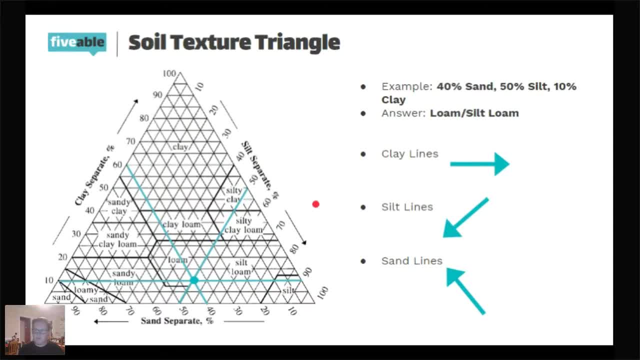 we have an example. so we have 40 sand, 50 silt and 10 clay, all right, so all the all the lines here. so if we go to this is what percent? 40 sand and we go up here or no, sorry, yeah, 40, yeah, 40 sand is going up here and then the 50 silt is coming down. 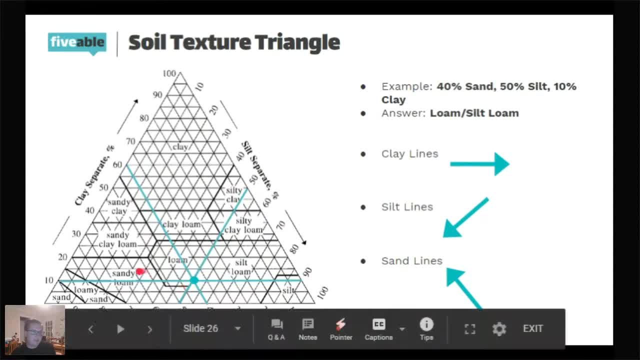 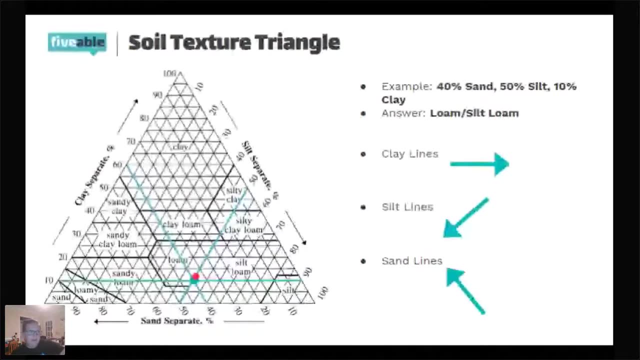 this way, and then the 10 clay is coming across this way, and then this section right here is is right on the line um. this blue line that's coming down this way is covering that up, but it's on the border between silt loam and loam, so 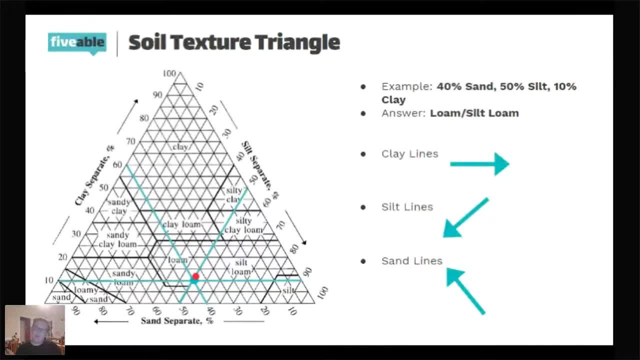 silt loam basically tells us there's a little bit more silt than the rest of them. but i have a question. so if it's silt loam, never mind, i won't ask that, never mind, all right. all right, so now it's your turn to try. um, what type of soil has 60? 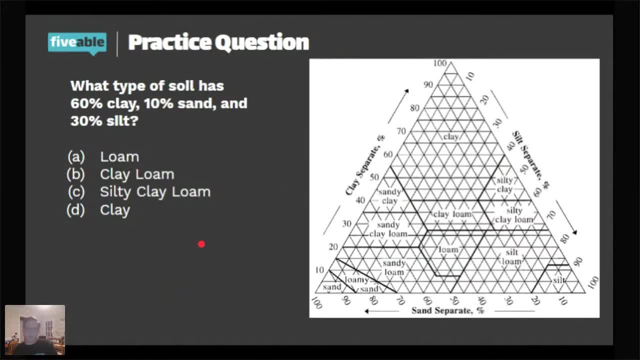 clay, 10 sand and 30 silt in the chat answer. i know it might take a while because it's on a computer, but on the exam you should be able to write on the stuff, so that should make it easier. um, are you guys confused on this question? 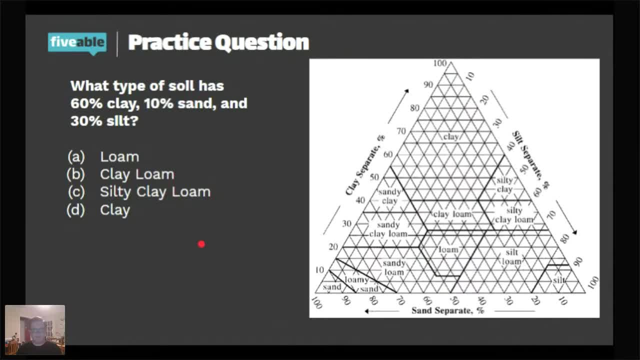 a little bit. no, all right, i just didn't know if you guys weren't answering. all right, you guys got an answer, maybe a guess, okay, and then look, a little harassment. i don't think you're familiar with what that is here. um, all right. um, okay. 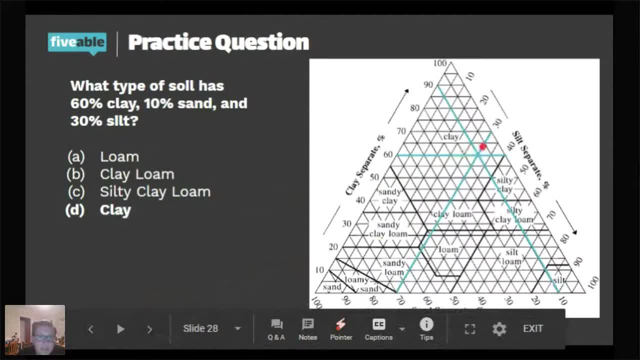 so we have clay, 60 percent clayline, and then we have 30 silt here inn here. wait, hold on, that's not on. see ShipMaker Lamb Roof Log arrive monthly this week, fine, um, um, whoops, um, um, um. Do you guys understand why? Because, remember, the clay lines are going this way straight across. 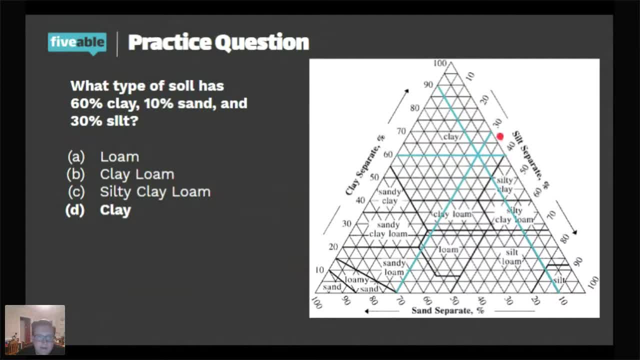 And then the silt lines are going down from 30%. So we already have the intersection here. So what I would do is I'd have the intersection here. So I already have the intersection between 30% of silt and 60% of clay. So the only thing left would be 10% of sand And, as it is here, 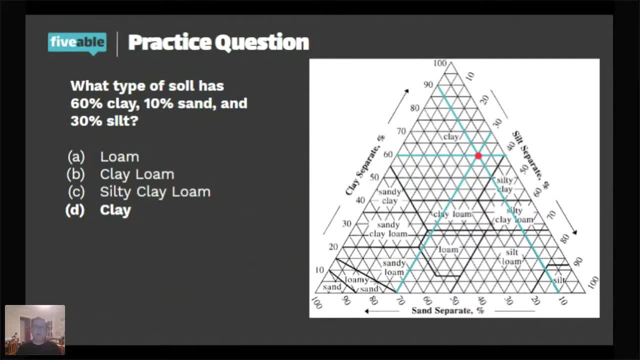 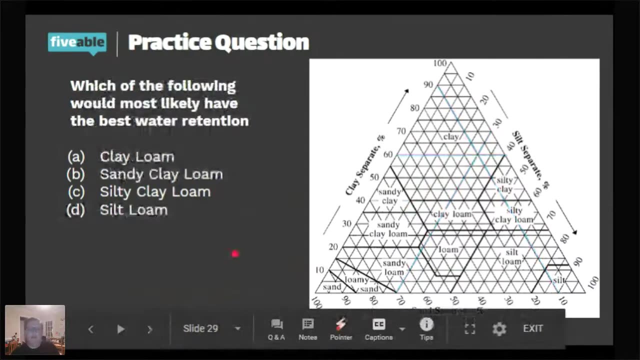 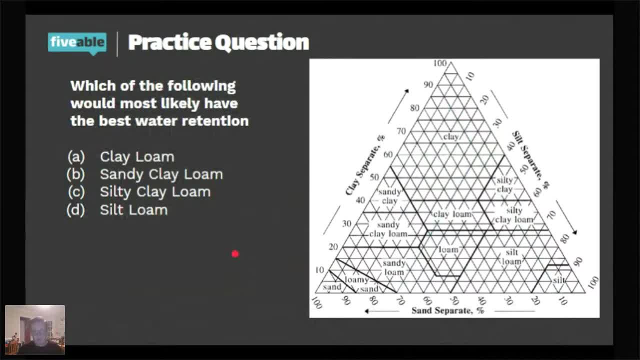 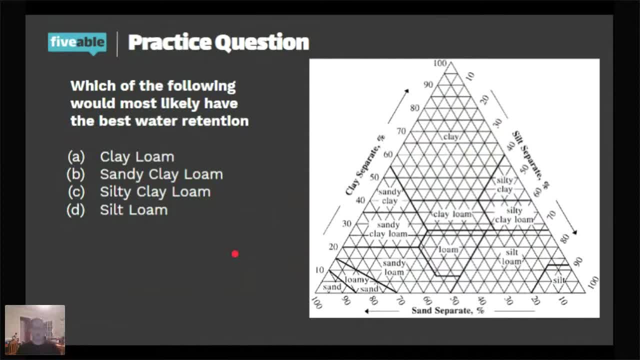 So the highest percentage of clay. Remember, the clay lines are the ones that going across. See now a couple of minutes to answer. give it a sip of water. I want some water. Right There you go. Yeah, Okay, so we have C-A-C-A. Okay, you guys are changing up your answer. Okay, so we say silt. 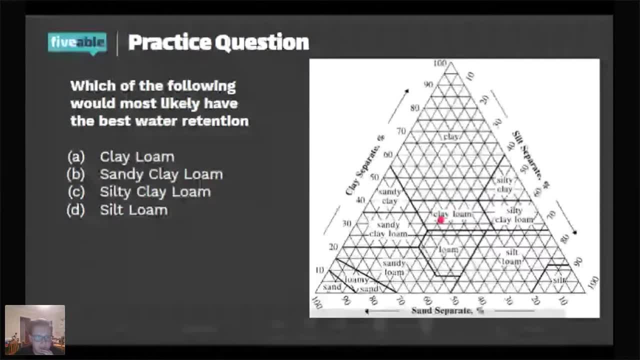 so: A- you guys said clay loam and then you guys change your answer, so we know it's not. B, because sandy clay loam is way over here. C is silty clay loam and then silt loam's. 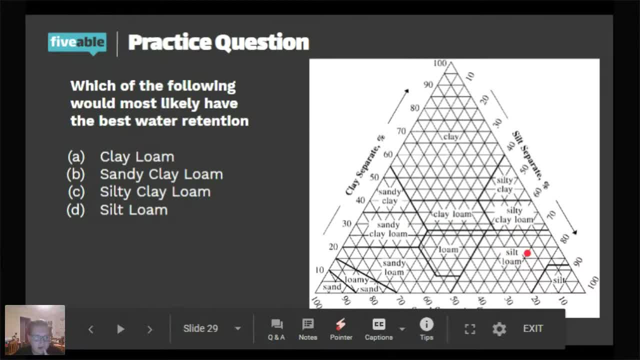 down here. So actually it could be C or D. Oh no, never mind, sorry. sorry, I was looking at the wrong lines. Yeah, it would be silty clay loam. Yep, No, because it's going across Silty clay loam. So something I have to really stress. 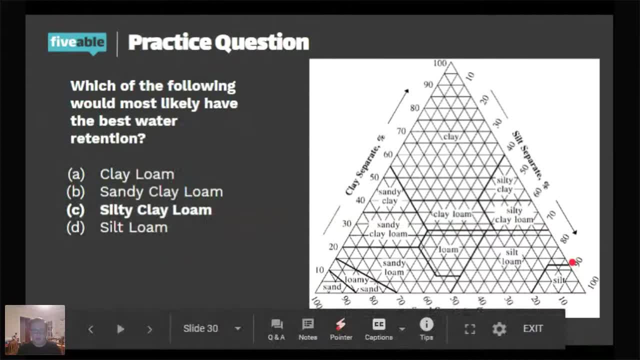 to you guys is: try not to get the lines mixed up, because that's what I keep doing, because there's like lines everywhere. So just remember, even if you get one of these on the test, just draw it out, Draw the arrows, just put clay, draw the little arrows over this way. 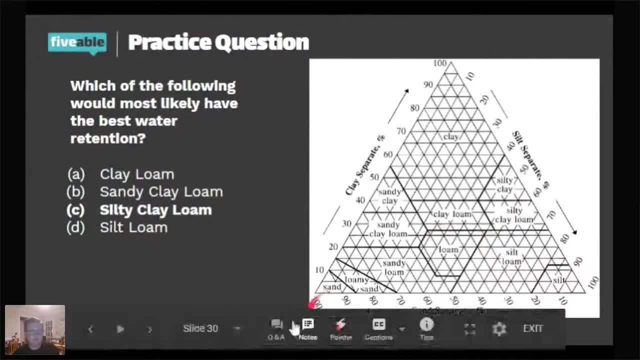 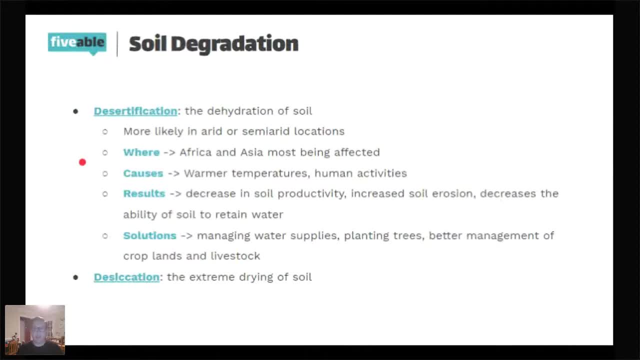 silt down or just follow the numbers, All right, So now we're going to go a little bit into soil degradation, and then soil and biomes, and then we'll be finished, All right. so first thing is: any questions with the soil? 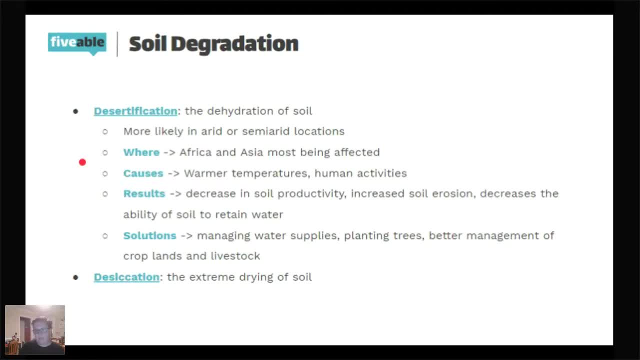 triangle, soil texture triangle. I can pull it up and we can do more examples if you want. You guys feel pretty solid on that, One through 10, how do y'all feel Need more help? So the clay goes down diagonally. 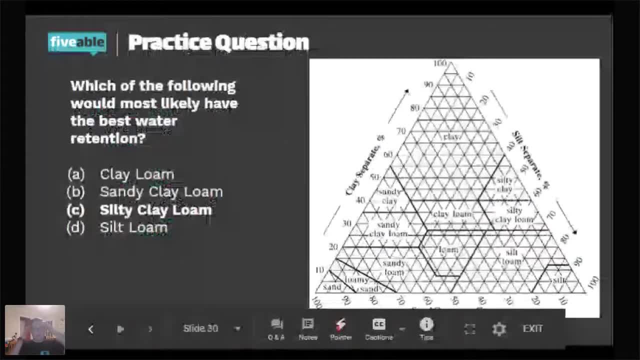 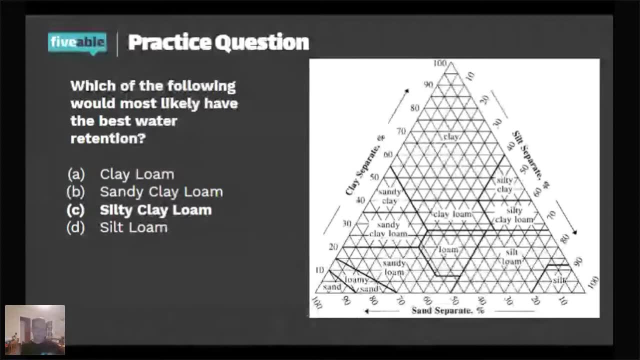 The soil goes across. I know it's hard, It's really hard. So the numbers? So if you look at the numbers, the numbers are straight. So it's just that way. Now, on silt the numbers are going down this way and on sand they're going up that way. Does that make sense? Yeah, 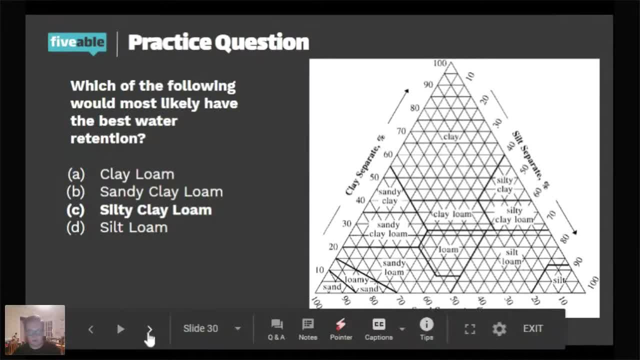 All right, Sounds good And if not, then just let me know and I can help you. Yeah, The same way, because more clay, more water retention, more sand we have, porosity and permeability is greater and stuff like that. So, yeah, this is all the same stuff. 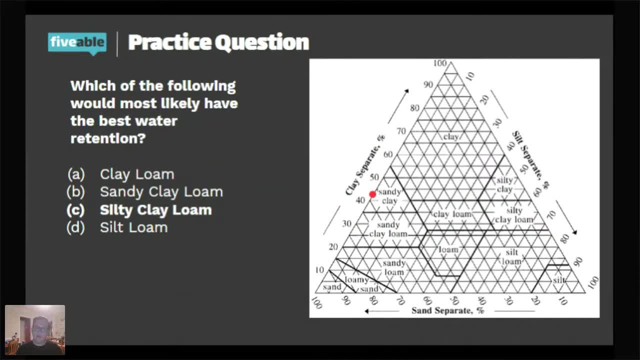 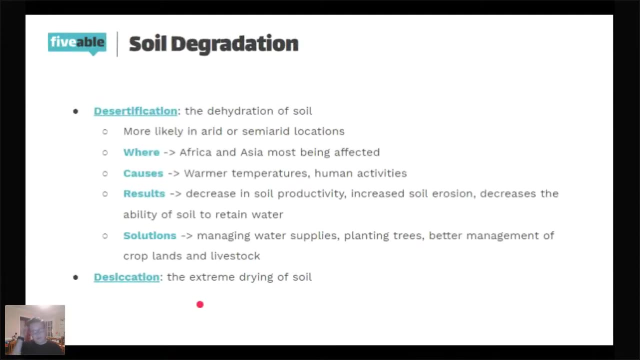 Silty clay. So it's clay with a lot of silt in it. Sandy clay: We have sand and clay Stuff like that. Yep, Just like we did earlier. All right, So the first type of soil degradation that we have is desertification. What does? 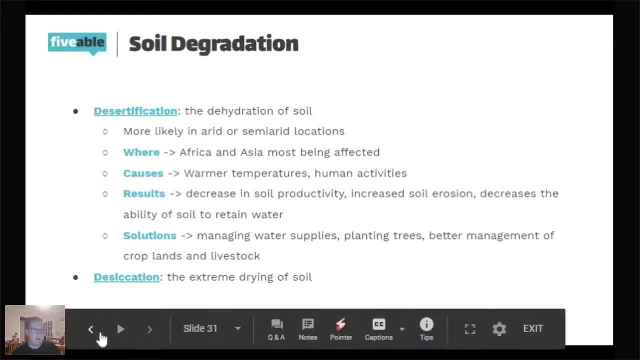 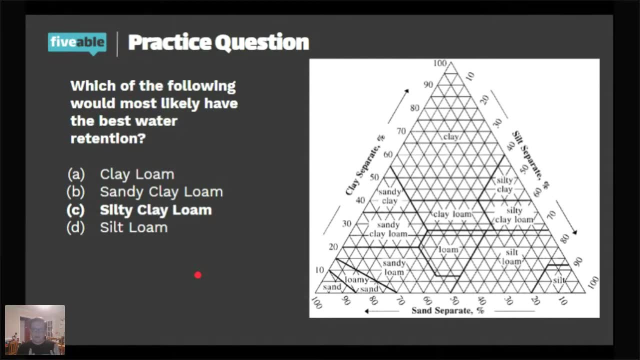 the clay separate mean- Let me go back, Okay. So clay separate basically means we took a sample of soil and we separated this amount of clay from it. So it's the- I think about it this way- The percentage of clay separated from the soil. 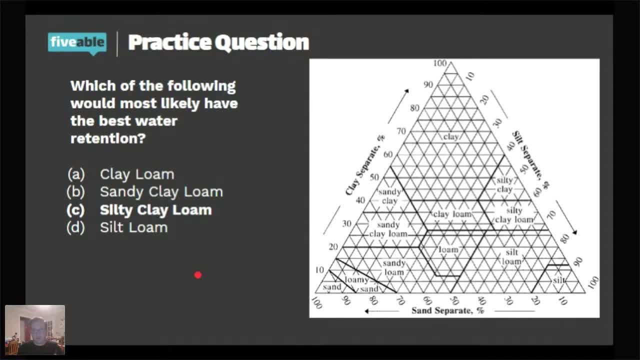 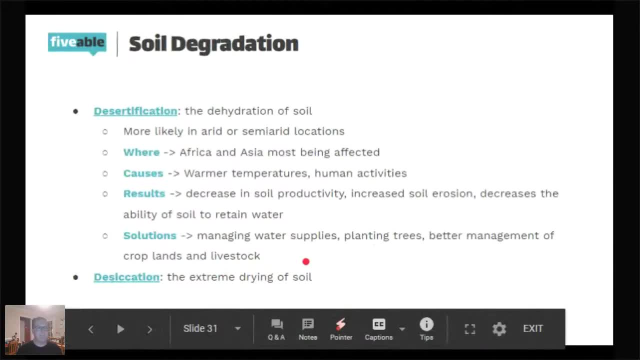 And then again for sand: separate Yep. All right, Any last questions, And it's okay if you have them. I want to make sure you guys get this because I know for me. All right, You guys got it. No, you do not have to draw it out, You do not. They will give you the chart and you will. 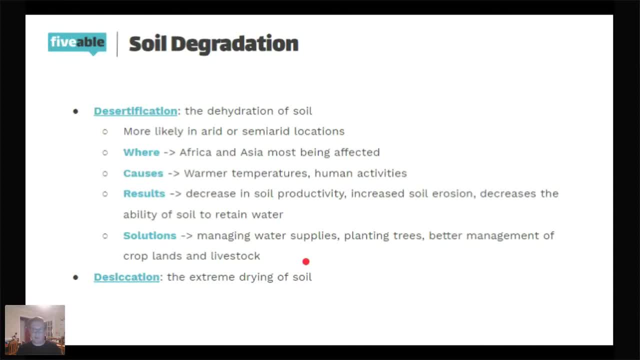 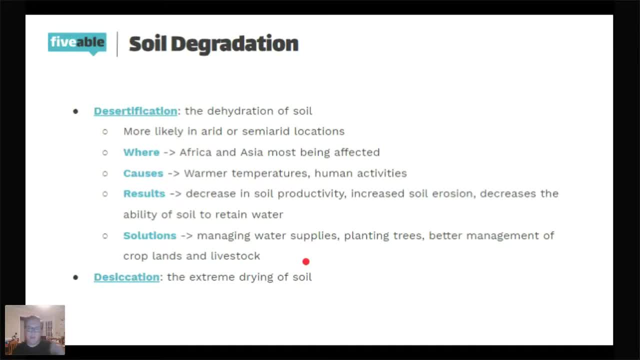 home. Don't go memorize the whole thing. Have the chart and they will just give you percentages. All right, Desertification: Basically the dehydration of soil, So this is more likely to occur in arid or semi-arid places. Basically, a lot of the water is removed from soil. 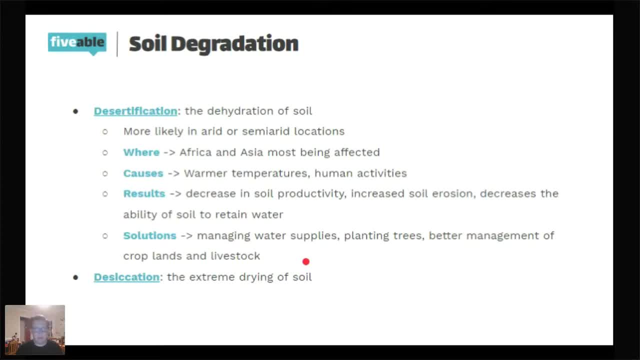 Africa and Asia are more likely to be affected by this due to their warmer temperatures. This can also happen from human activities such as logging. if you think about it, Trees and plants- they're going to hold the water and the roots better. 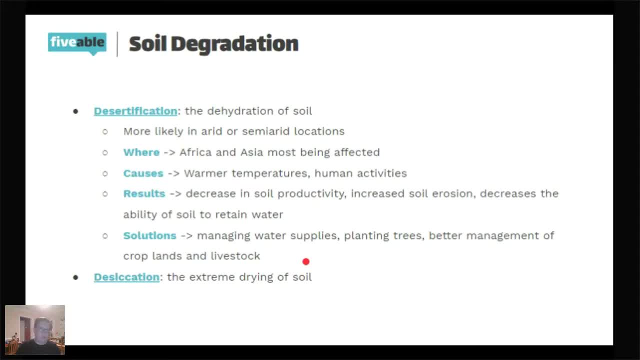 So if we take the trees out, then water and nutrients are more likely just to flow out of there. Result: decrease in soil productivity, which is an obvious one, That's soil degradation. Increased soil erosion. we have this dry soil easily breaks off. 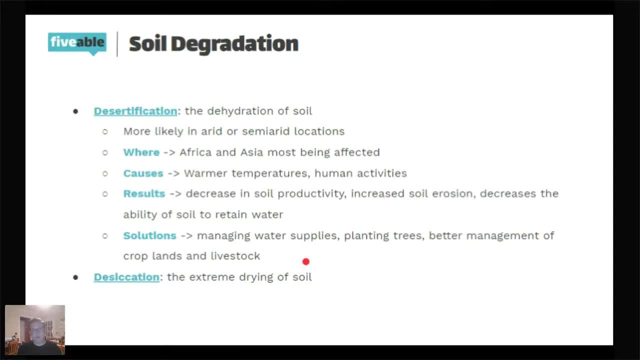 And decreases the ability of soil to retain water, which might be negative to our plants. Solutions managing water supply, particularly like if you have crops that take a lot of water. you might want to plant less plants that need less water or more irrigation. 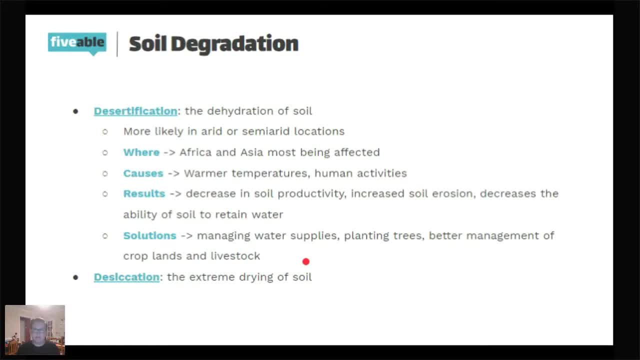 Planting trees And better management of crop lands and livestock Grazing if your animals are eating up all the plants. And then there's another thing. Now, this wasn't on the CED, but whenever I was in AP Environmental Science we went over it. 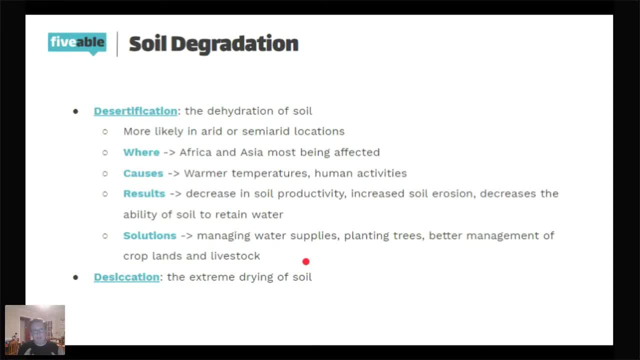 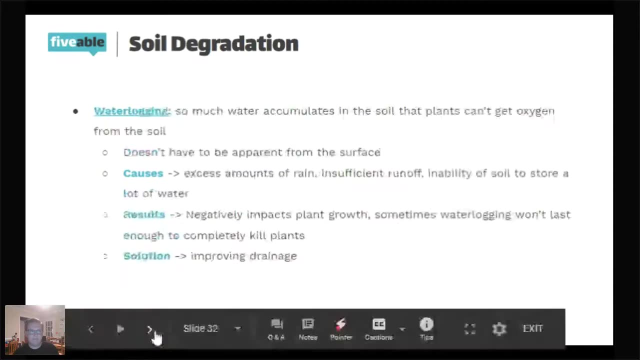 It's called desiccation, which is basically desertification, but worse. So it's like extreme drying of soil And you're going to think: the same consequences and causes but more extreme. And then we have waterlogging, which is basically the opposite of desertification. 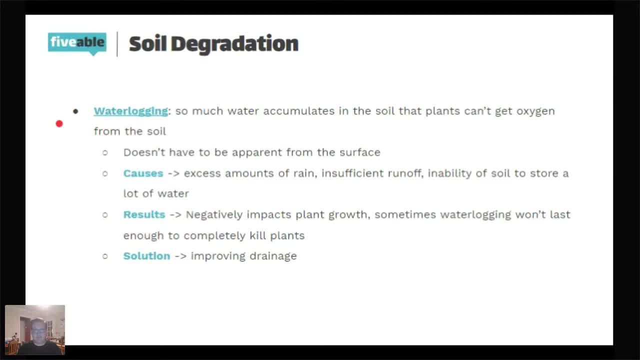 Basically, so much water accumulates in the soil, the plants can't get oxygen from it. It doesn't have to be apparent from the surface. Sometimes it can be more underneath, a little bit lower underneath the surface, But this can definitely happen if you get excess amounts of rain. 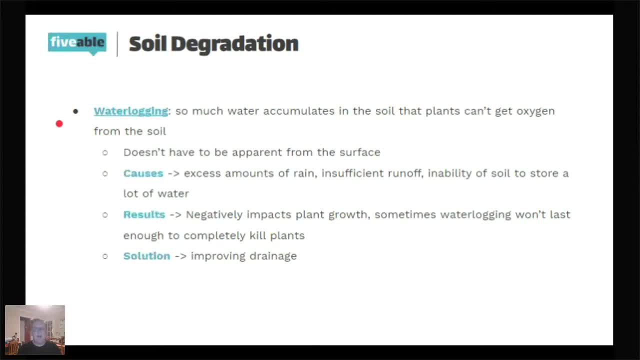 You've probably seen it happen. You go out. puddles are starting to form in the grass. That's an example of this Insufficient runoff. You might have a lot of irrigation going into like a crop field or something like that, But unless the water has a way to get out, you're sort of kind of trapped there. 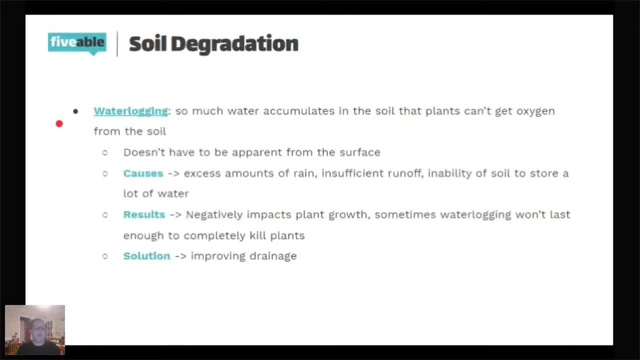 Inability of soil to store a lot of water. At first this one confused me. I was like: what do you mean? it's storing a lot of water, But it's like, I guess, like there's not enough room, I guess. 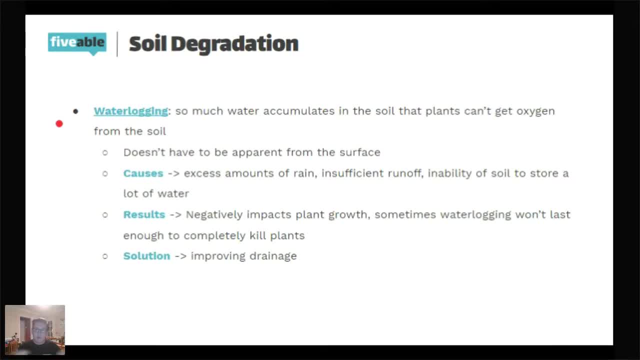 It can't store a lot of water, so it starts puddling on top And ultimately becomes a lot of water. Results: negatively impacts plant growth. However, this isn't as intense Water logging won't last truly long enough to kill plants. 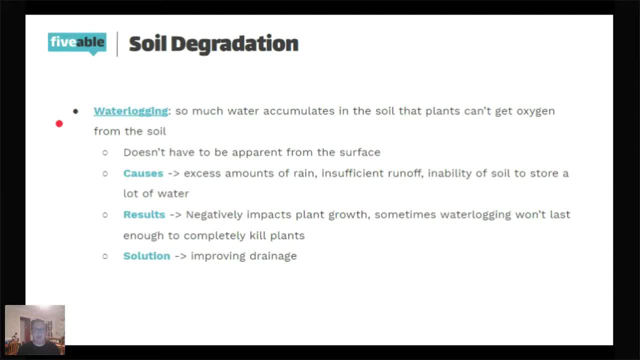 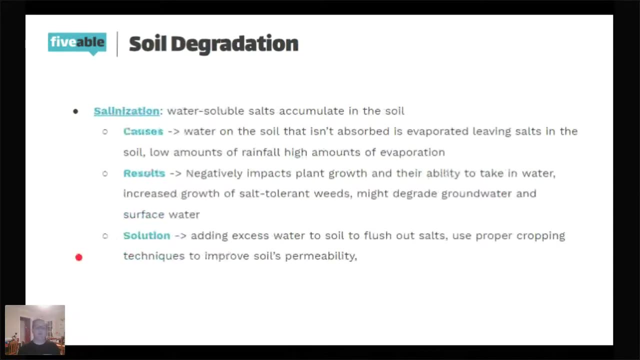 And the example I used before: rain: building up. eventually it goes out, But the main solution here is improving the drainage. Because you have a lot of water, you need a way to get it out. Solidization, So basically water soluble salts, accumulate in the soil, causes 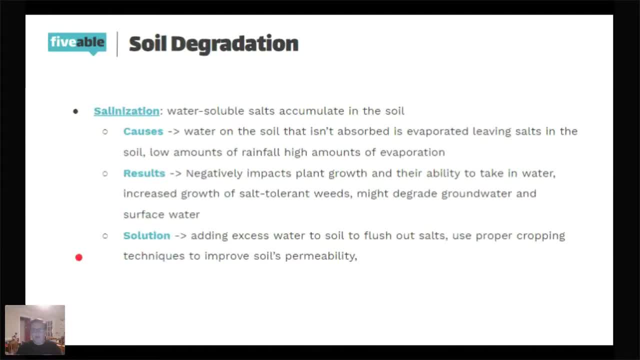 So like think acid rain and stuff like that. So acid rain is coming down on the soil but it's not absorbed, So it's just sitting on top. So this might be like a water logging type situation And then it evaporates and leaves the salt on the soil. 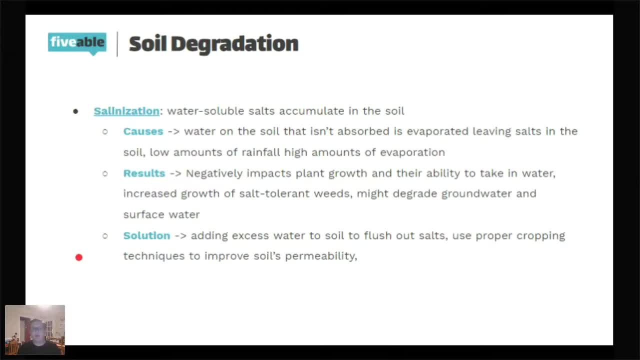 That's why it doesn't evaporate, But also so, basically, low amounts of rainfall, high amounts of evaporation. So, like any water, It's just being evaporated and leaving salts. This can negatively impact plant growth And take in their ability to take in water. 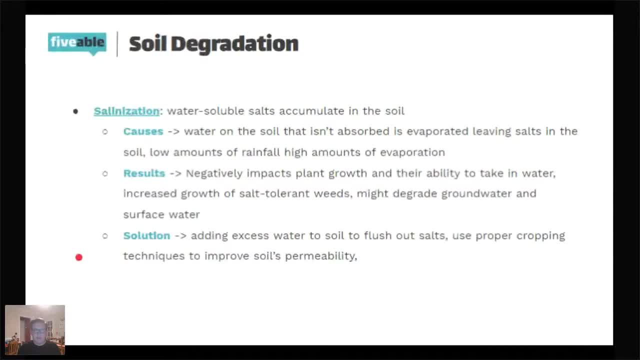 Because, if you think about it, if the plants Are taking in the salt Yeah problem, We have increased growth of salt tolerant weeds and also might degrade groundwater and surface water. So It's important to keep these salts out of the soil. 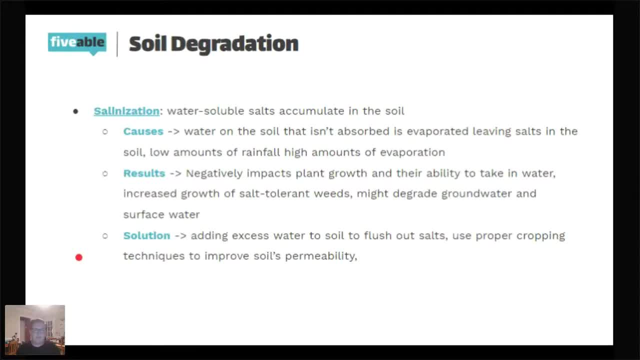 So that doesn't get into the water, So that doesn't get into the water table. And then, finally, the solution is adding excess water To the soil to flush out salts. Use proper cropping techniques to improve soils permeability. So make sure you're plowing and turning up the soil before you plant, and 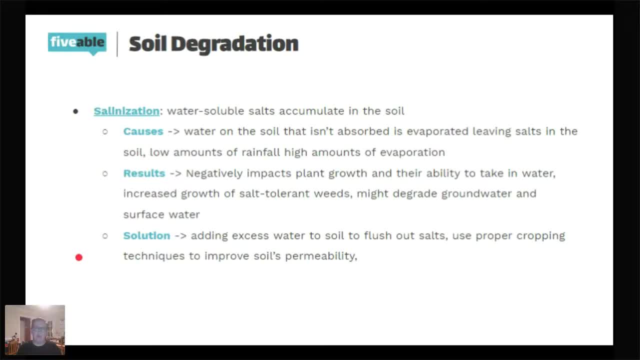 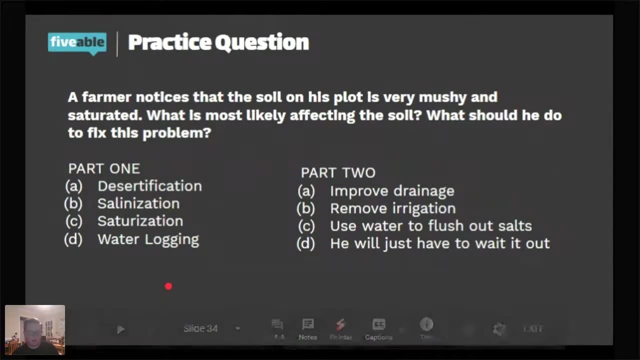 all those other Things- I'm not a farmer- Some of those things that I'm not a hundred percent sure about. but turning up the soil, All right. Any questions? Any questions? No, I went through that local Fast. 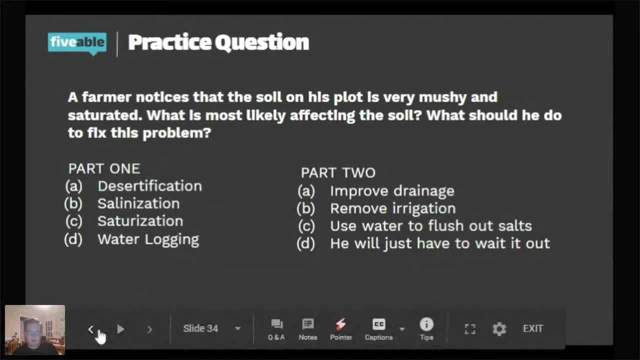 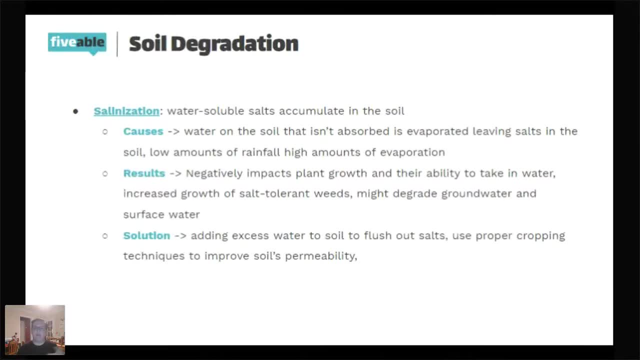 Acid rain come from beaches? Acid rain doesn't come. I don't think so. Acid rain usually comes from when released pollution into the air like smoke and stuff, And then it reacts in the atmosphere and mixes with water And then it comes back down as rain with the compounds. 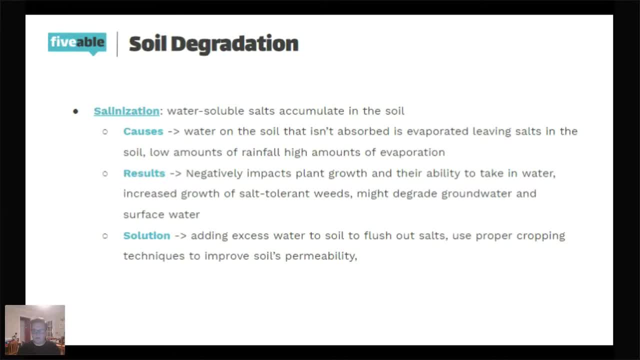 with the water And the compound together, Yeah, And then that falls And the salt In the water Evaporates and leaves the salt on soil. But you can also think solidization and desertification Might have some correlation, because the salts 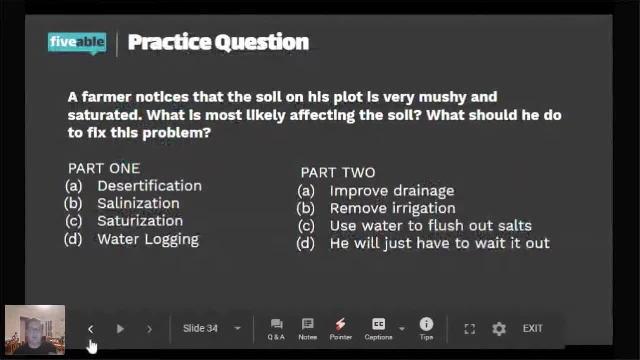 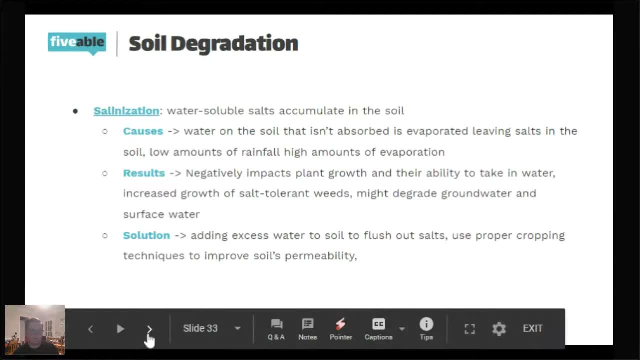 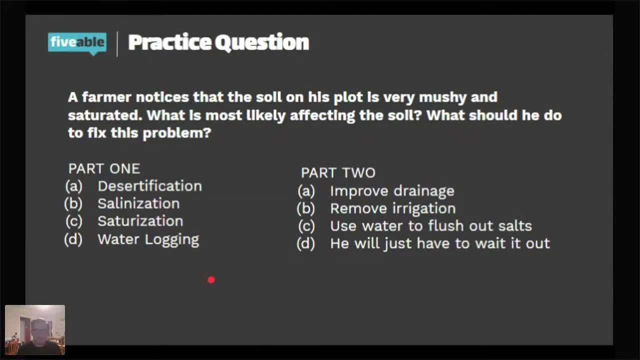 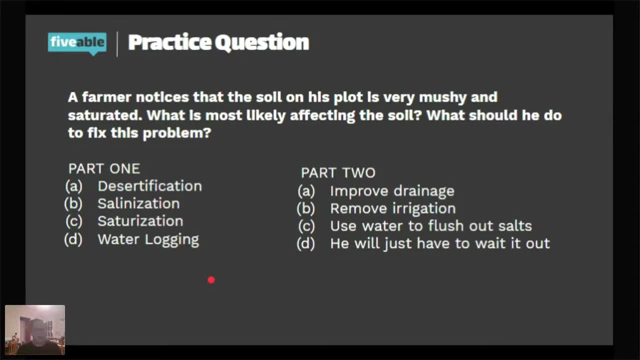 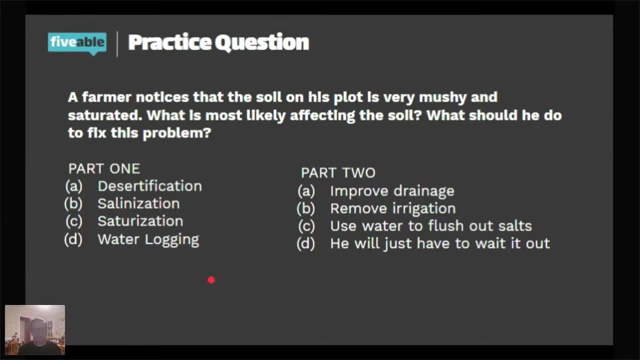 Improve drainage. B- Remove you. C- Take water and flush out salt And D- You'll just have to wade it out. Yes, Yes, So Water logging, excess water floating up in the soil, and then a you want to improve that drainage. 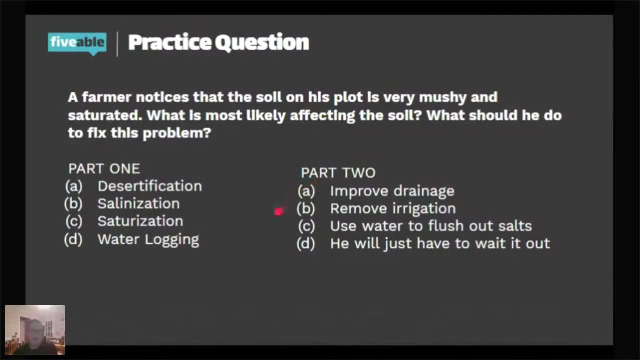 to flush it out. but it might also be D on the second one because, remember, in the case, like the rain that cause might cause water logging, you just have to let it go. so so those are two things that you could do is wait it out or improve. 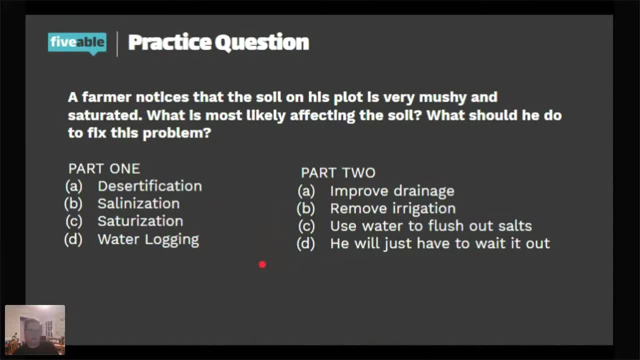 drainage it depends on because, like, if it's chronic and it's just like water logging, it has really rained that much, or it has rained so much that there's so much water has to drain it out, or you can just wait it out for like a rainstorm. 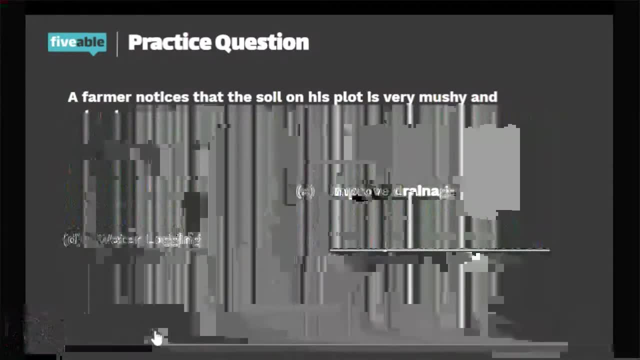 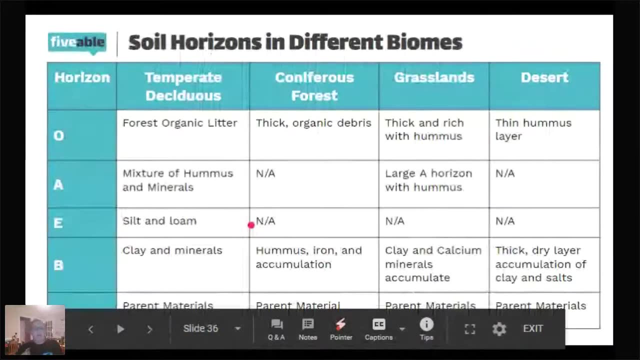 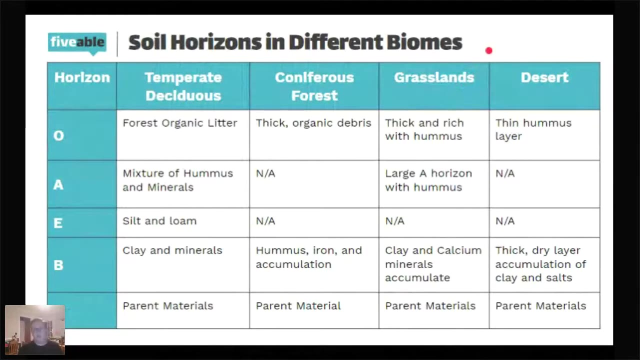 that brings a lot of rain. that's why that one's underlined yep, all right, so this is a little bit about the soil horizons in different biomes. I think, Sarah, you said you wanted to look at this. it's definitely um, I mean, it's not the CED, but I think it really helps you sort of kind of. 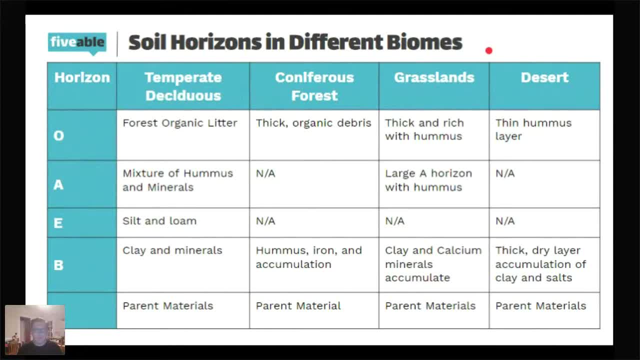 understand exactly what these layers mean. so if we look here- I have notes here, all right- so if we look at a temperate, deciduous forest, we see again the forest, organic litter, which is the leaves, sticks, all the decaying organic matter, and then a. okay, so a is a mixture of hummus, which is that organic material. 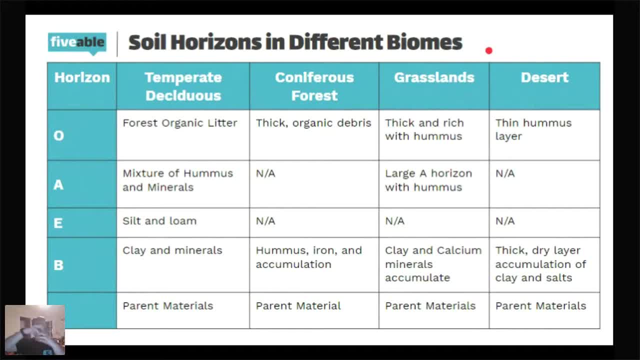 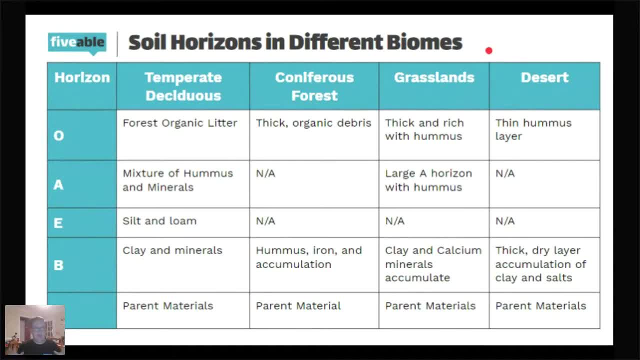 low, which is the good balance of the clay, salt, silt or sand sand, not salt, um, and there's sort of kind of mixing there. and then remember, e is that транс zone of leaching where the nutrients are going down into the B horizon, and then 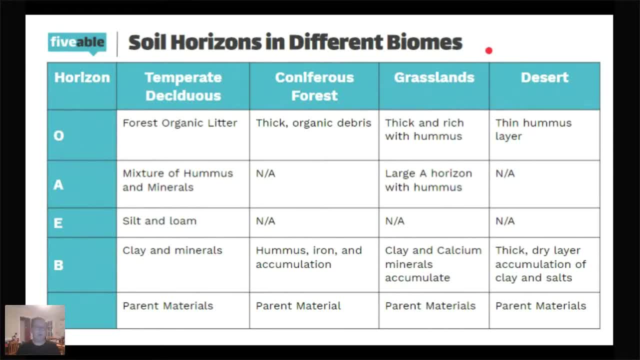 is that trance zone of leaching where the nutrients are going down into the B horizon B. we sort of see the clay and minerals building up And then C is parent materials. But she's going to be parent materials for a lot of them because basically it's just the broken down bedrock. 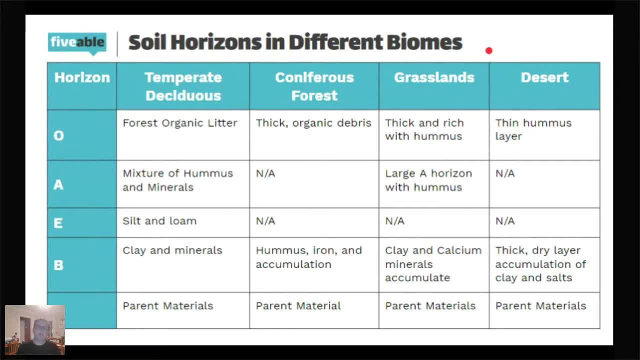 which sell all soil forms Right. Another thing to note is that all of these, like all these layers, might not appear, Like you might have, like a big layer and, let's say, coniferous forest, a big layer. It's like all together. 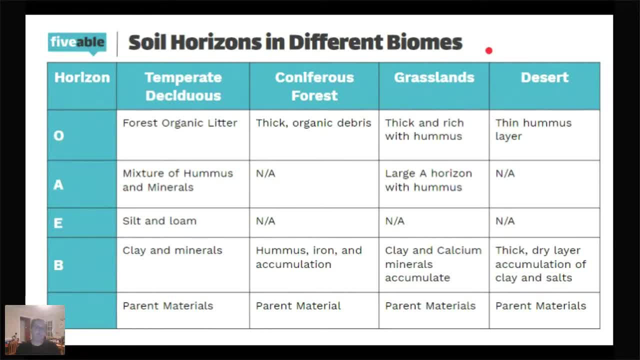 Not that there's one So, and that's what we have. So our O layer is thick and organic debris And then, like our B horizon sort of kind of makes up for the A and E and then the O, It's more, you have less horizons, basically. 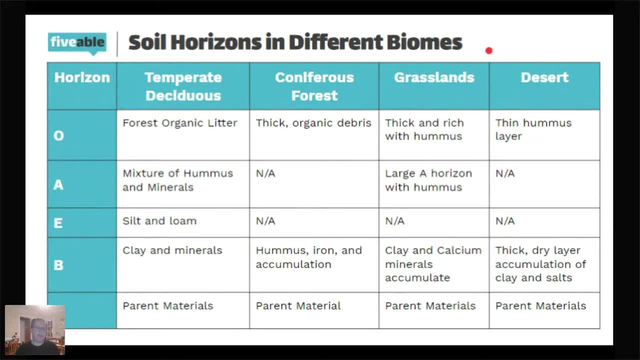 So in our A, E, B sort of kind of mixture here we have hummus iron and iron. hummus iron and I think it's supposed to be aluminum accumulation There are. remember the E is pushing these minerals down. 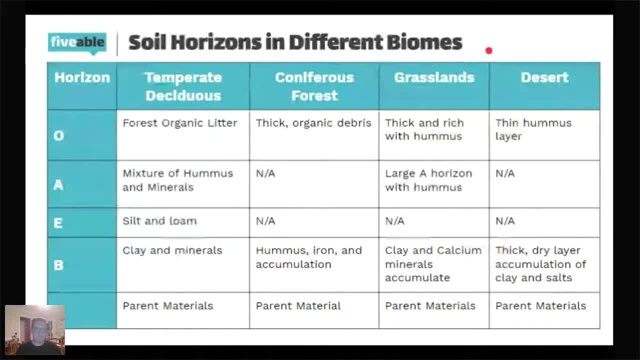 They're accumulating in B because the parent materials is bottom. and then grasslands. if you remember- I think we did a live stream a couple of months ago- Grasslands are very productive, with plants thick and rich with hummus, So they have a pretty decent O horizon there. 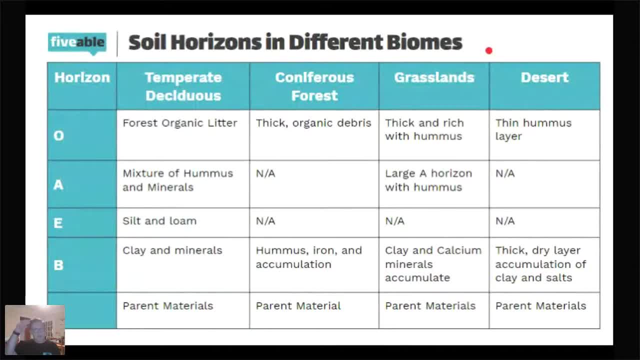 They have a large horizon with hummus. So it's like whenever I looked at the picture it was a pretty decent- excuse me, I'm out there. And then E: we really don't see E, but B we're going to have. 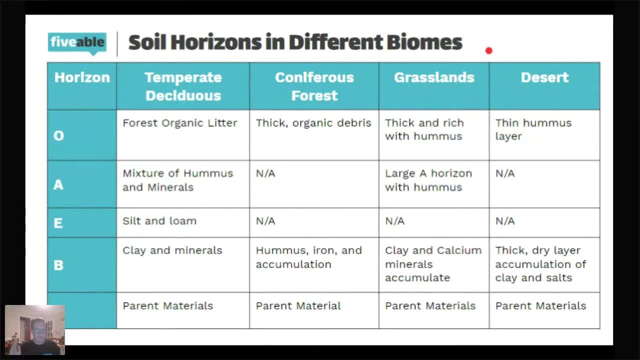 remember that's where all the stuff accumulates. B is where stuff accumulates: Clay and calcium minerals accumulate. and then C is parent materials. Just think B is where everything accumulates because it can't go further down, It can't go down to the C horizon. 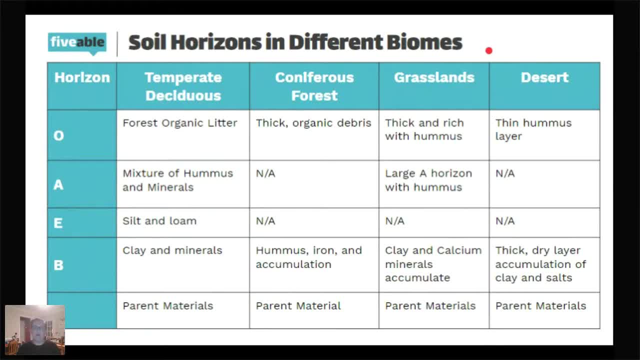 It just doesn't work. Now. O remember the question we had back there. We have the thin hummus layer that's up there And then really the A and the E right here. I don't know- I'm trying to point to it, but A and E. 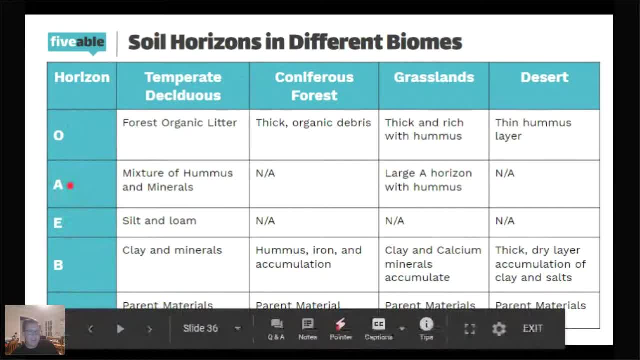 they're both like A and B, they're all one. So we see basically a thick, dry layer, accumulation of clay and salts. Yeah, so that's what majority of the sand is. And when they say, thin layer of hummus, which is like the good dirt, 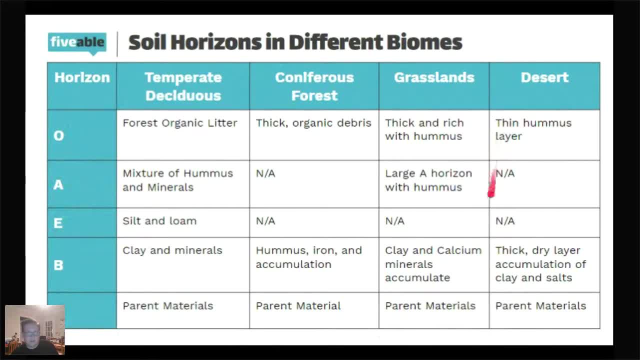 I mean like very thin, like sometimes they won't even have it, And then parent materials, And then also, when you're doing, when you're thinking about different soil horizons, different biomes, you can also think about what the biomes like, like the tundra. 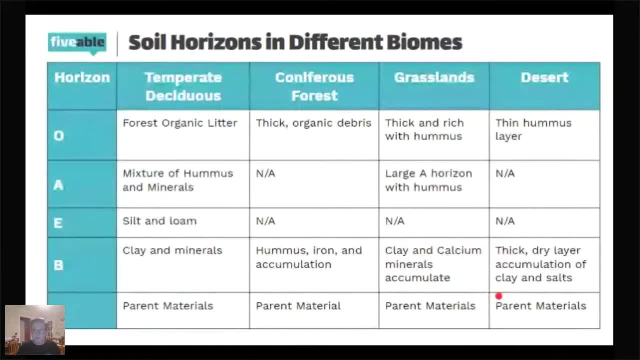 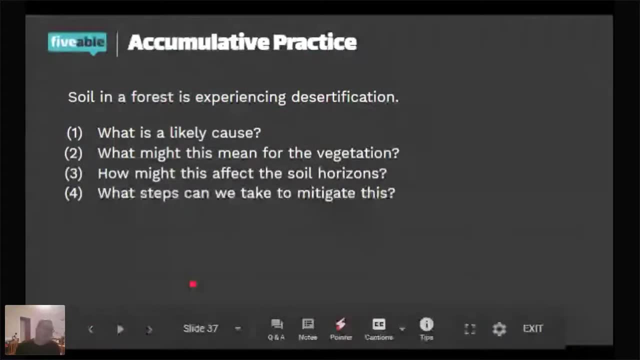 It's not on this PowerPoint, but you can think about it. They have the term frost soil underneath You can think. so we're kind of use your knowledge to think about what might be in these different soil horizons. All right, soil in a forest is experiencing desertification. 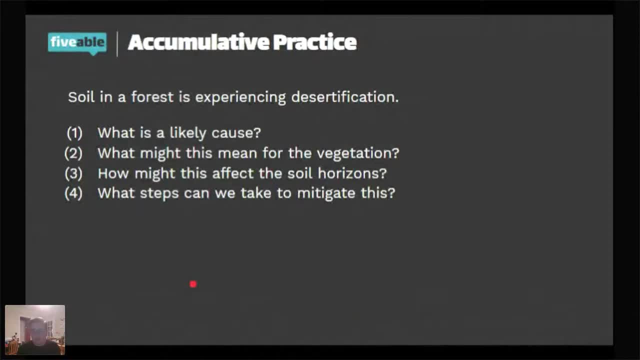 Number one: what is the likely cause In the chat? let me know what is the likely cause of this desertification? Too arid? yes, We also have logging. Remember the trees are keeping the, keeping the water and nutrients there. 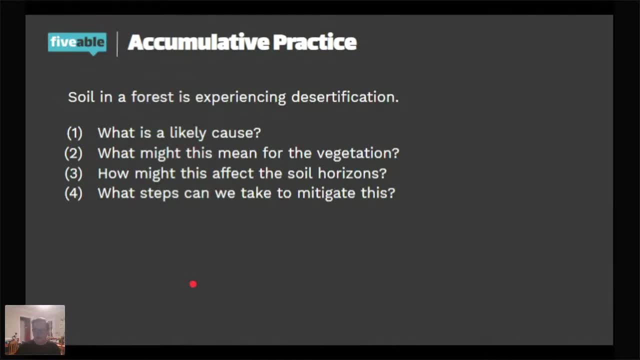 So if we're logging and taking all the trees out, then the water is just going to be able to flow right on through Two. what might this mean for the vegetation there? Desertification, Less plants- Yes, They're going to start to die off because they don't have the 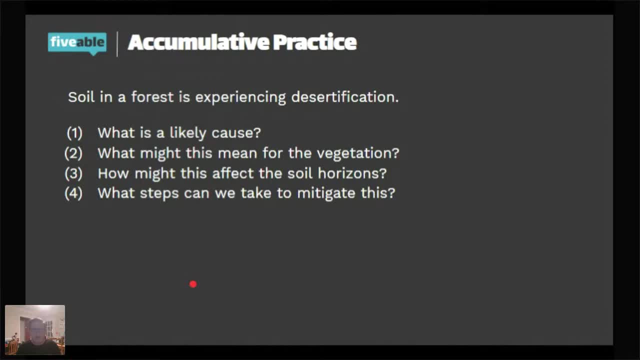 and plus they're already going to die because the trees are dying. So, yeah, so the plants are decreasing. Um, vegetation is dying because they don't have nutrients or water, which really that's like, if you think about it, they need vegetation to hold that stuff in there. 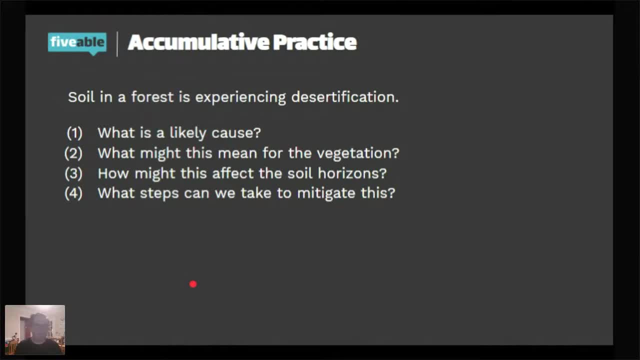 But when you take away the trees and it just starts dying. so we're kind of like a feedback loop. All right, So three, how might this affect the soil horizons? Yeah, O horizon is going to go down and also the hummus is going to go down, because 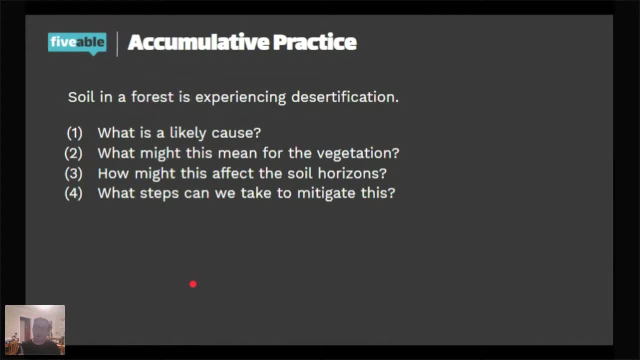 and now this is over time, Like at first the O horizon might actually go up a little bit cause we have all the plants decaying, but after that it's going to go down cause we don't have a lot of biological factors breaking anything down. 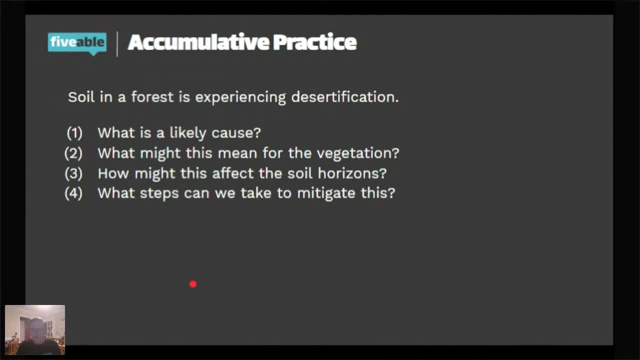 We don't really have anything decomposing. We'll still have an O horizon. everything's going to start to be dry, Um, like the desert. it's going to start looking like the desert horizons: more dry, less nutrients, Um, and for what steps can we take to mitigate this? 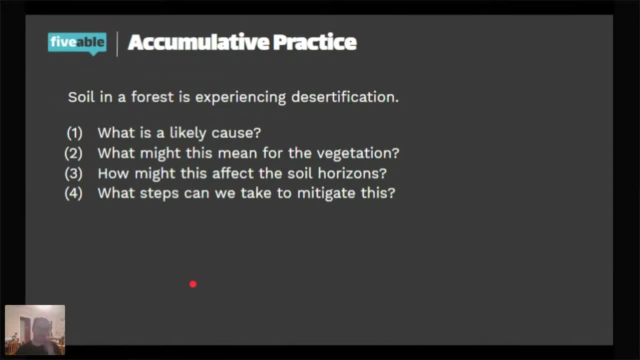 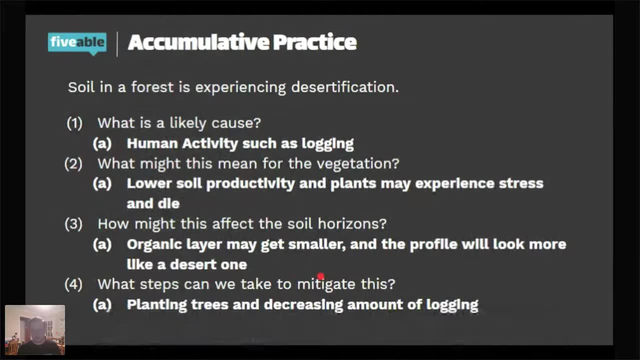 Yes, Water, um, add water, Oh gosh, Um water. planting trees. decreasing the amount of- yes, irrigation planting trees. decreasing the amount of logging that's happening to get the plants into the ground to hold everything there too. 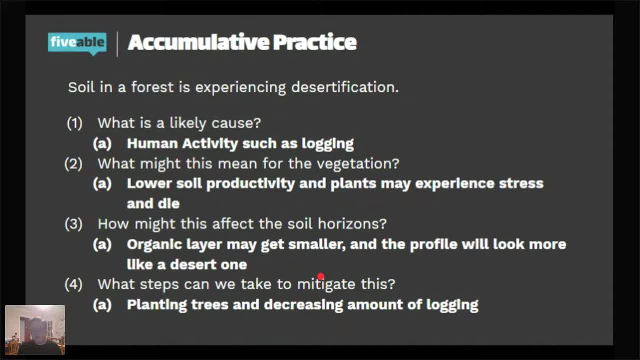 Cause, if you irrigate it, um, what else? I mean like that's a great solution for it's working like a in the moment type solution, if you get what I'm talking about. Um, but again, really just, we really need to also plant stuff too. 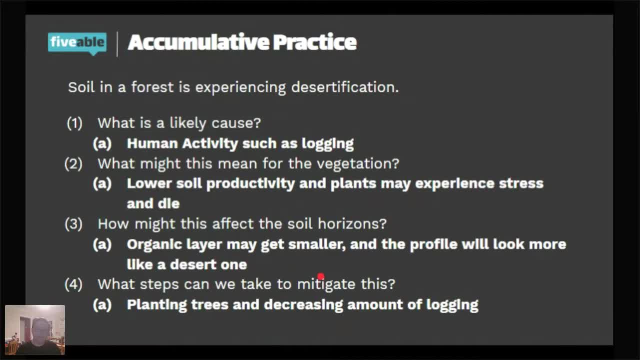 So I think irrigation and planting trees and plants is works great together, cause you're holding everything there, All right. Well, that is it, guys. If you have any questions, let me know in the chat. Um, we can go over the soil texture triangle. 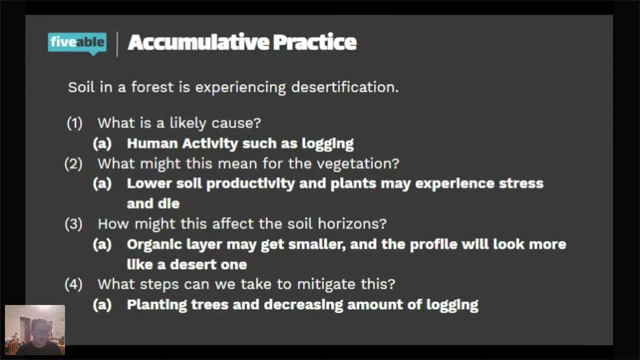 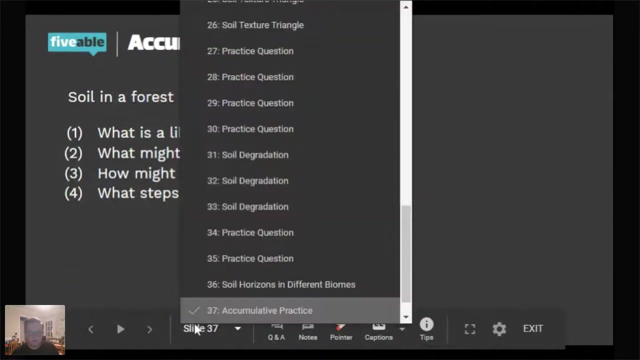 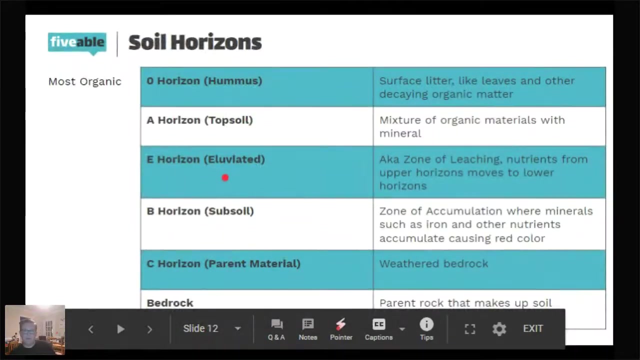 If you have any questions, soil horizons, if you have any questions, anything about soil, I can answer. All right, What's the difference between the B horizon? All right, Go back, Okay, Between the B horizon and which other horizon and the A horizon. 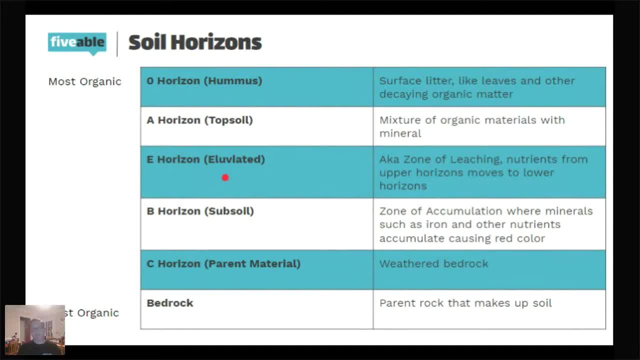 All right. So in the, in the A horizon is sort of kind of the boundary between, like, the E and the O. So from the O we have surface litter it's coming down and we have minerals that are coming up from this parent, from the parent material down at the bottom. 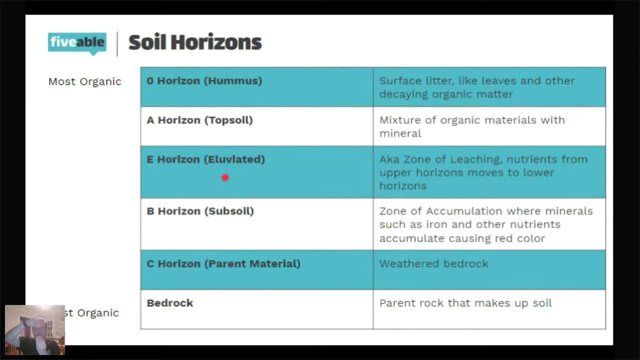 So that's sort of kind of where the A is very organic, rich cause near the top And it has some minerals in. Now the B horizon doesn't have the same nutrients as that topsoil. We see more like iron, metals, salt. 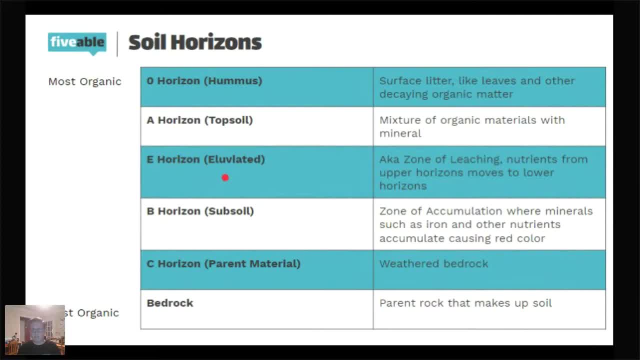 Oh, she mean another horizon. Do you mean the E horizon? Nevermind, All right, You got it Right. Well, this PowerPoint, Oh, keep going. Okay, So in the B horizon. um, okay, So in the B horizon. 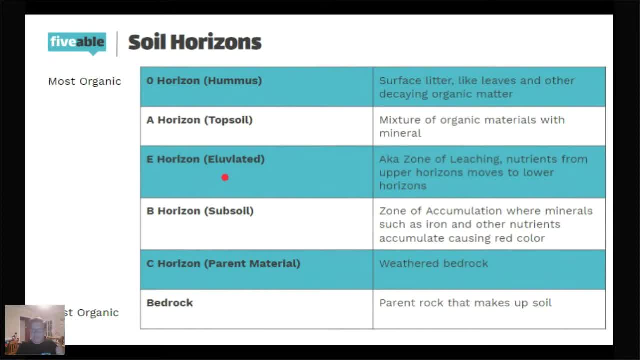 we're. they're not getting the same nutrients as the A horizon is. So we're getting more like metals, salts. We're coming down here. Um, we're not getting like like the nitrogen and oxygen and the carbon that's rich in the A. 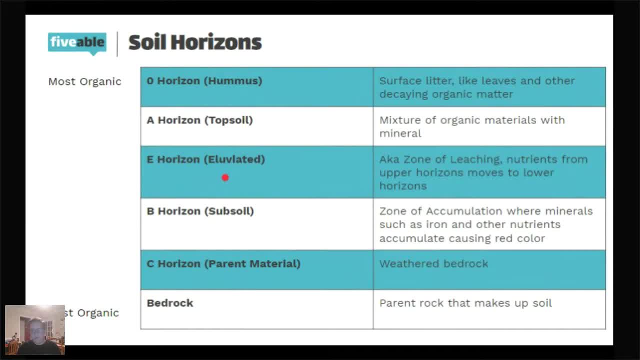 horizon Isn't really in the B horizon. That's really um, like iron, aluminum, clay, sometimes calcium, I know, builds up there. So basically they have different minerals, Okay, And then they're leaving another place and they're like: well, 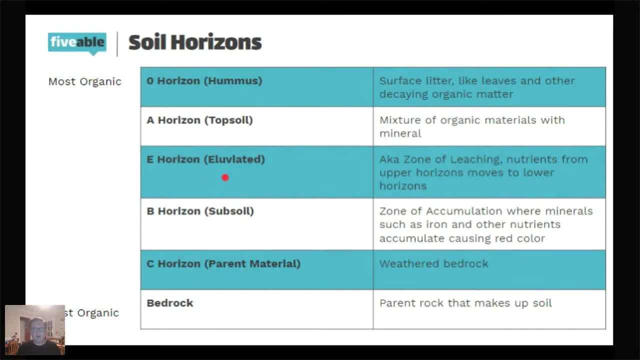 they're just not getting a lot of. they're not getting a lot of, uh, they're not getting a lot of nitrogen, Okay, So you know, I, I think I know this is a good place to end this, do Yeah. 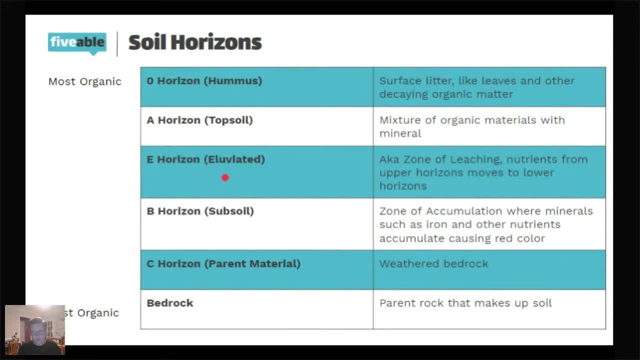 yeah, I think this is a great place to go, Because that that's that's an excellent question. It's a great thinking on a your mind And then we- I um- continue to. I think we're gonna have one or two more questions. 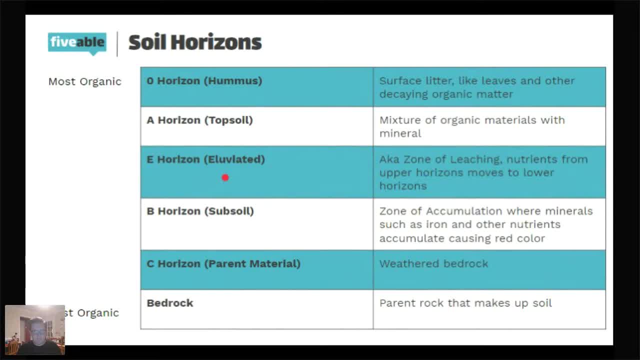 What's, um a good question. there's a question I'm going to ask now. if you have any questions, Um, I wanted to ask this question because I want to take that as a no for questions. Well, I have. what is C-O-N-F, Do you know? 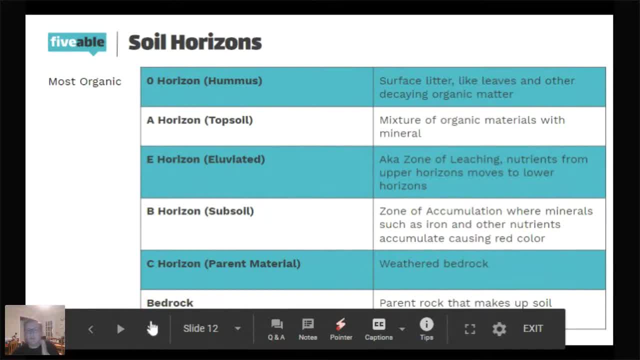 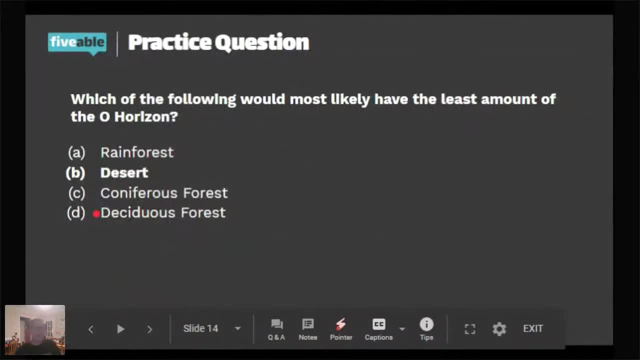 what slide that's on Coniferous. Coniferous really stands for okay, so coniferous are the cone trees, trees with cones. So if you think, like Christmas trees have pine cones on them, pine trees have cones on them. Deciduous forest- I don't know a good definition for.